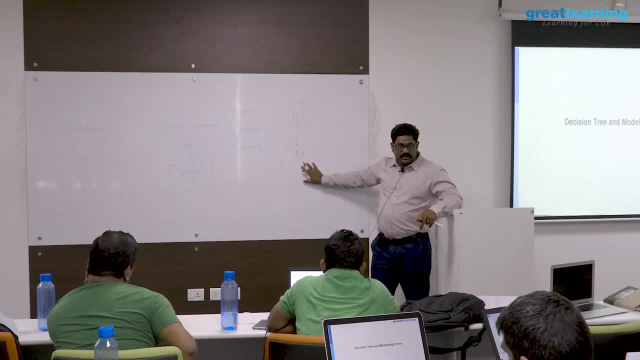 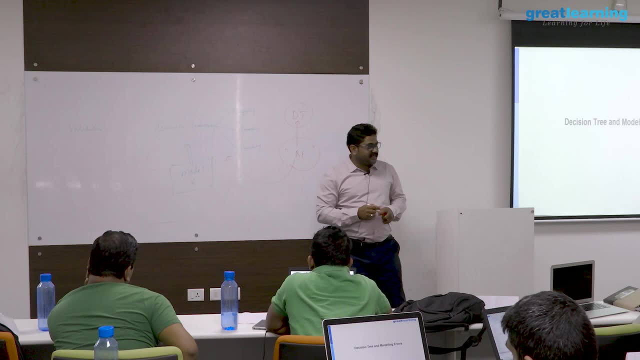 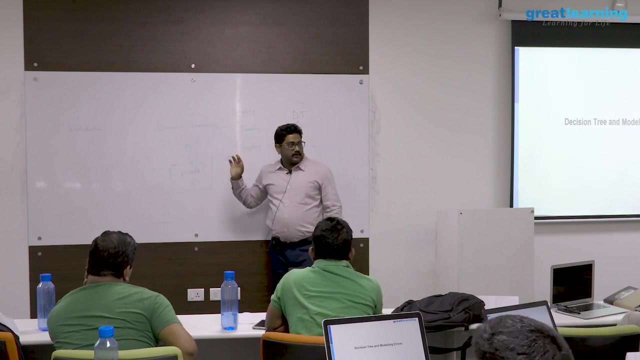 of decision tree, how the drawback is overcome by random forest. Ultimately, in turn, this random forest algorithm itself. among all the models you have listed out at the beginning, among all the models, whether it is a linear regression or logistic, SVM or KNN, whatever the model, we have to explicitly apply any of these techniques to 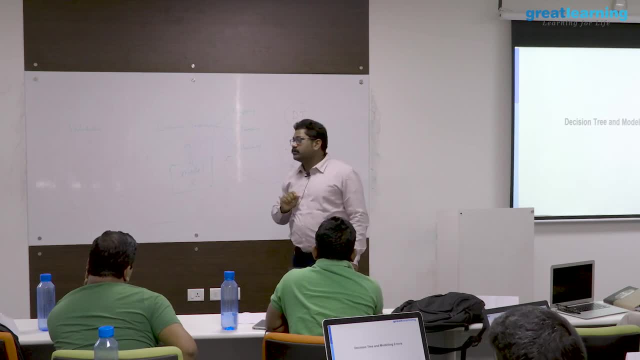 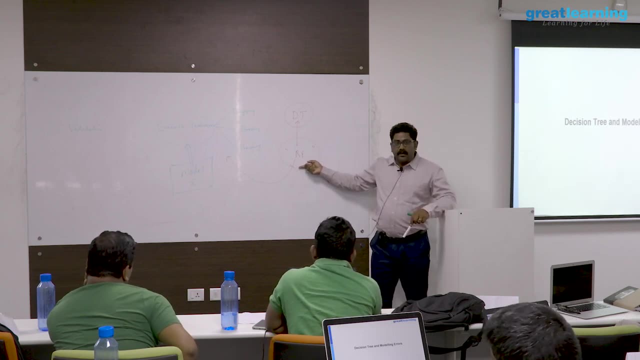 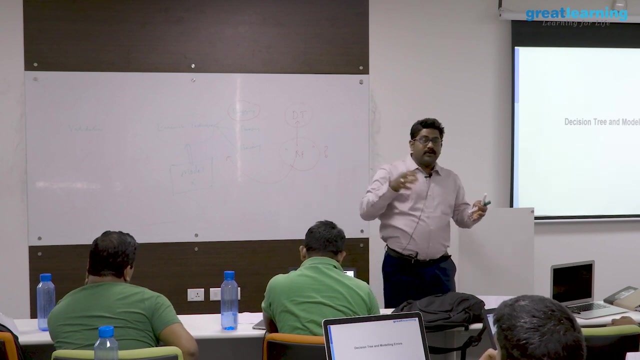 improve the performance of that model. except one model. except one model. That model is random forest. Why The question mark? why random forest? It is not needed because it has a built-in bagging boosting mechanism. not boosting mechanism, I will say built-in bagging mechanism. Any one technique or single model we know, we 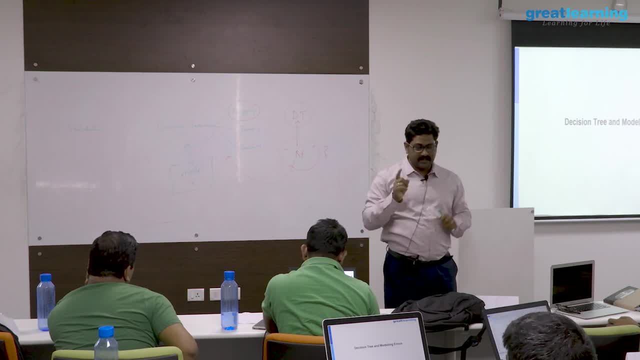 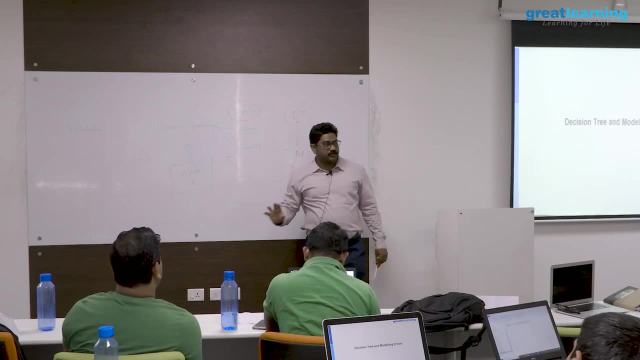 do not apply all three together. Please remember, for single model generally, we do not apply all three. Either bagging is one approach, boosting is another approach, stacking is another approach. Which approach is best suited for your data sets? you have to pick, Do not. 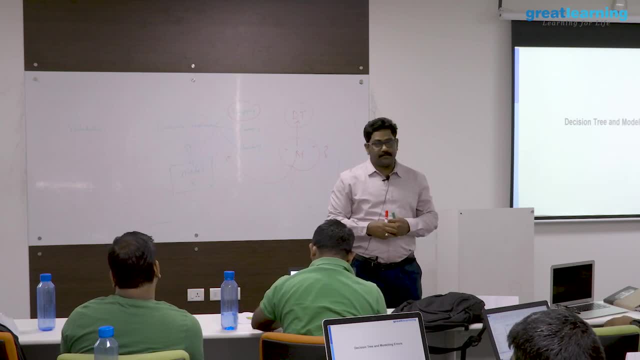 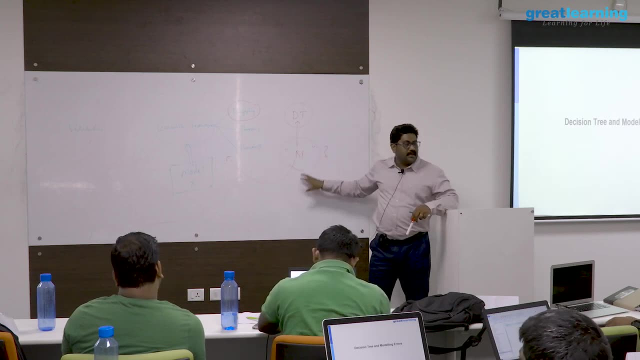 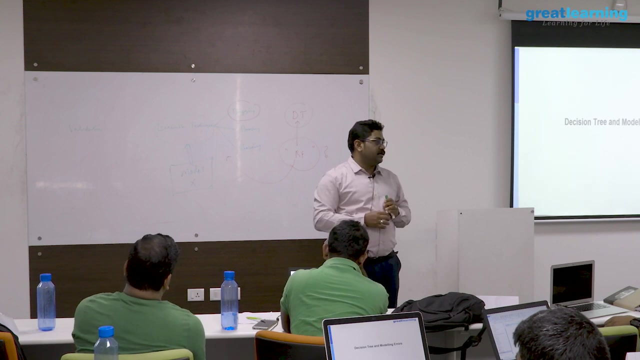 think using all three will give me the best result. No, Any one approach at a time Among that random forest. Why we are studying random forest under the ensemble category? Because the model itself has the behavior of self-tuning behavior. ensemble behavior. What behavior Out of these? 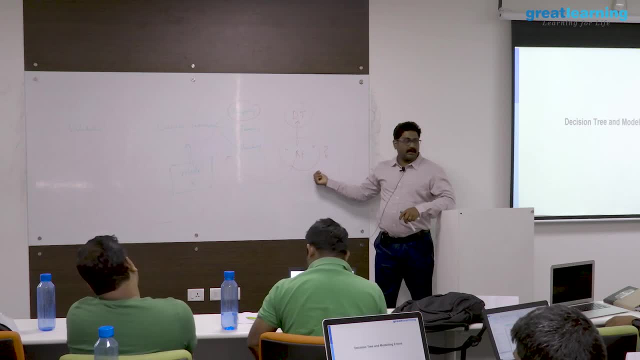 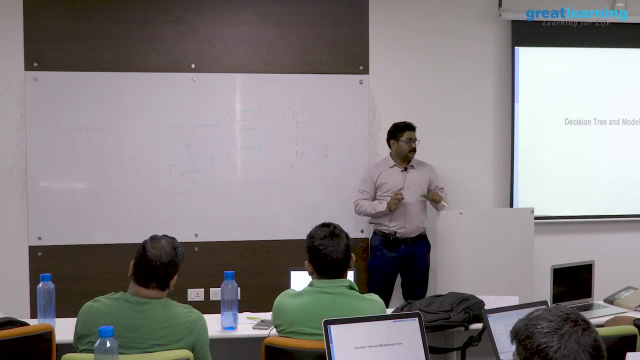 three bagging behavior. That is why we are studying random forest under this ensemble learning category. To appreciate that we have to start with the decision tree. To appreciate that phenomena, we are going to start with decision tree First. we will start with the decision tree. 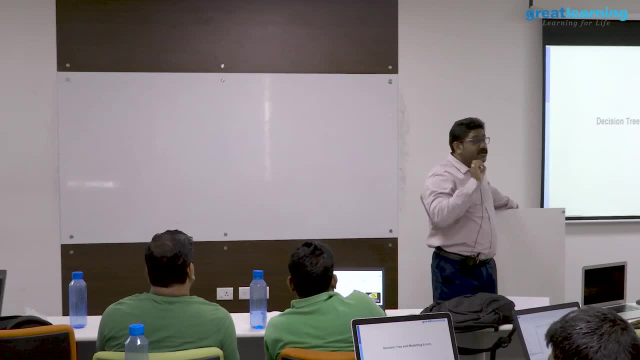 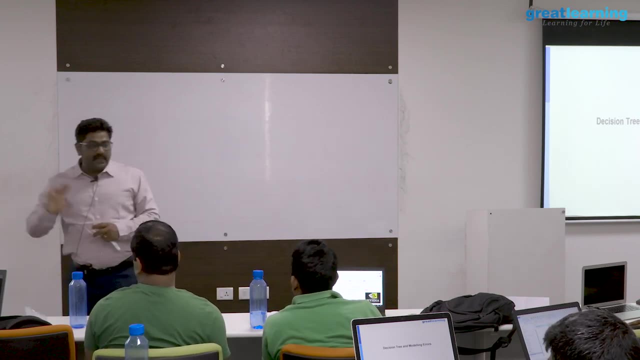 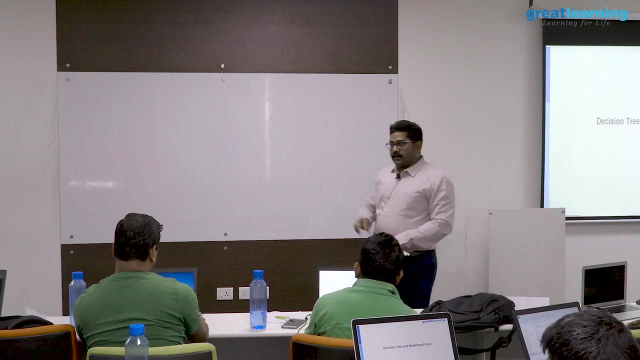 I mean to say that random forest the only one machine learning model which has the built-in ensemble learning capability. you got it, Whereas all other model explicitly you have to apply such capability either by doing a bagging or boosting or stacking approaches. Random forest is the only model it has the 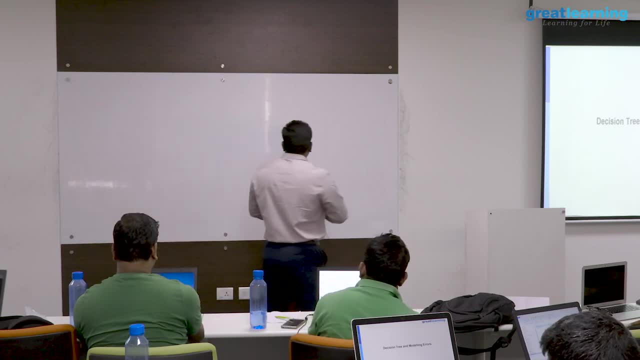 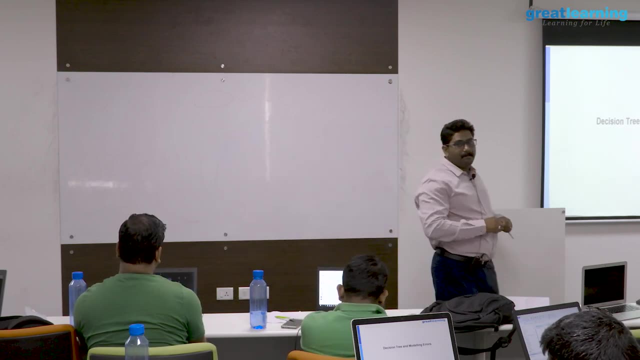 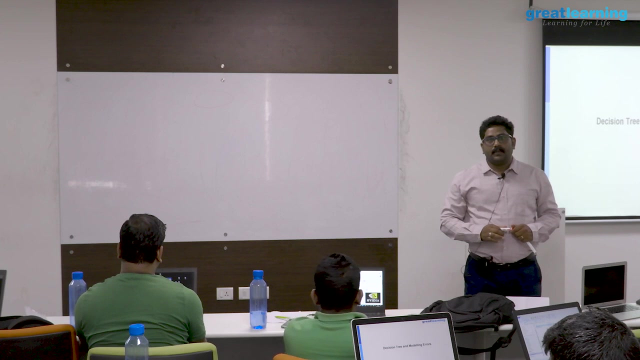 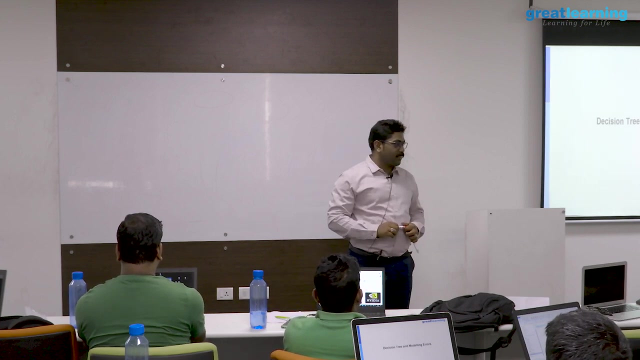 built-in capability. Decision tree is one of the simplest classification model. no complex math like SVM, SVM- among all the machine learning model, I could say SVM is the toughest Implementation perspective. all are equal, from sklearn, import, modelfit, modelpredict. anyone will do Implementation perspective. Understanding the background, math and stat I am talking. 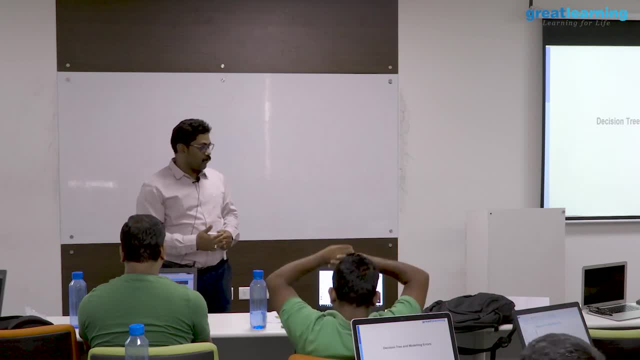 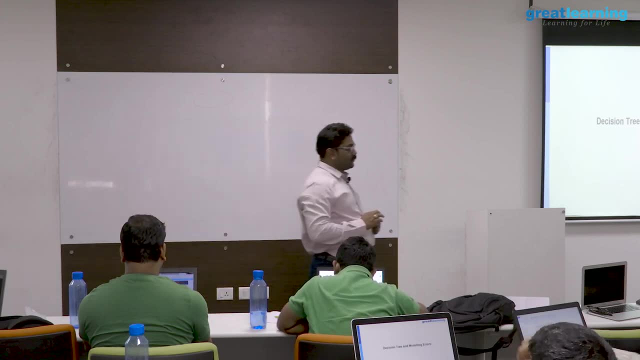 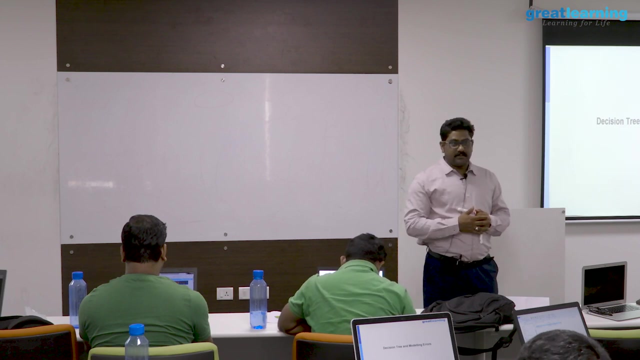 about Understanding the background, math and stat behind every model. SVM is the toughest Because understanding the kernel itself. it will take lot of time for you- Different kernels- to study about the different radial basis function, how RBF is working, how polynomial kernels is working. You have to deep dive on to that. So it has a depth of understanding. 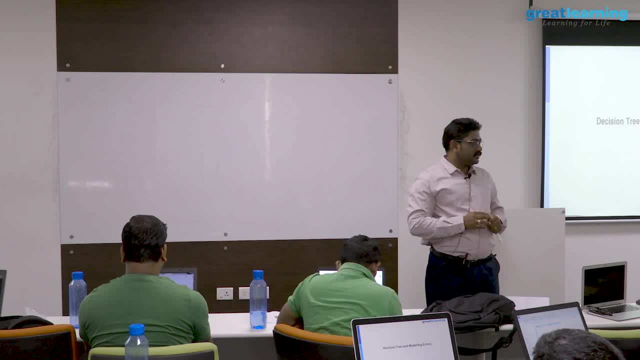 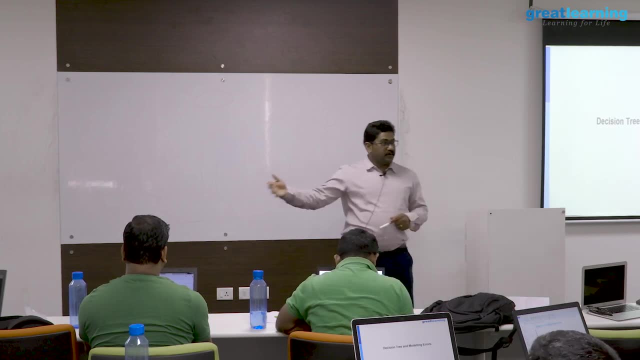 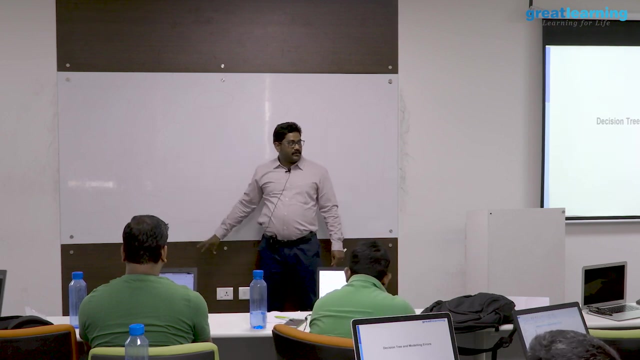 Generally people say neural network is the toughest of all the model. But truly SVM is the toughest to understand mathematically. Of course neural network also like why I am comparing that among all other model. You do not have such complex math involved in decision tree. It is a simplest of all. 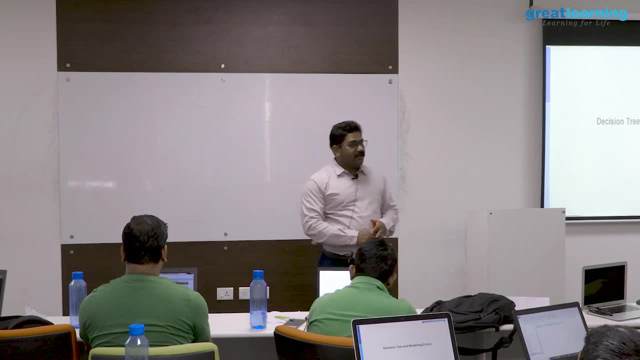 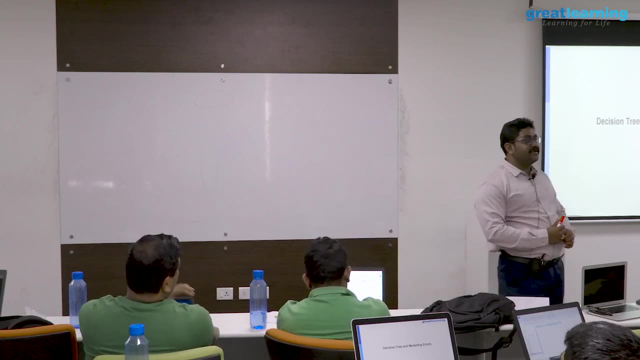 the models K-NN. you have started with K-NN, K-NN also, I can say K-NN. is there any complex math behind K-NN? Only distance metric. Any test data comes if you say 5 nearest neighbor. 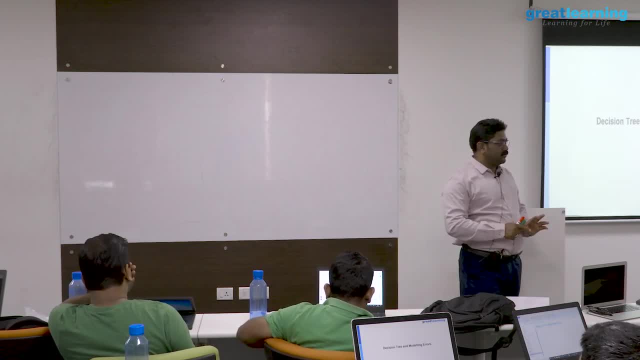 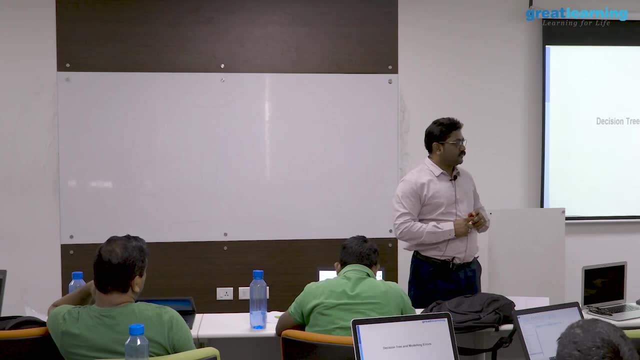 you calculate the distance to all the records, All the records. you sort it Closest to 5, you pick Among the closest to 5, you pick the who is the majority? Why we go with odd numbers: To avoid tie. To avoid tie: always go with odd numbers for. 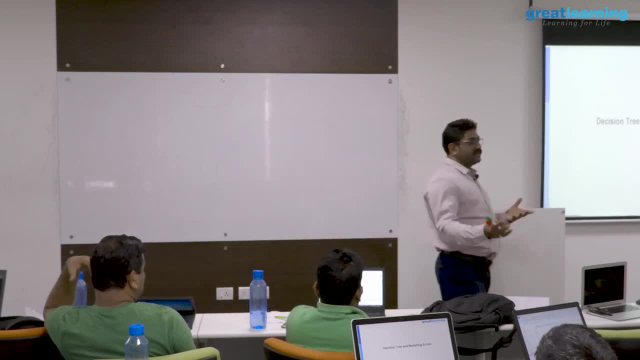 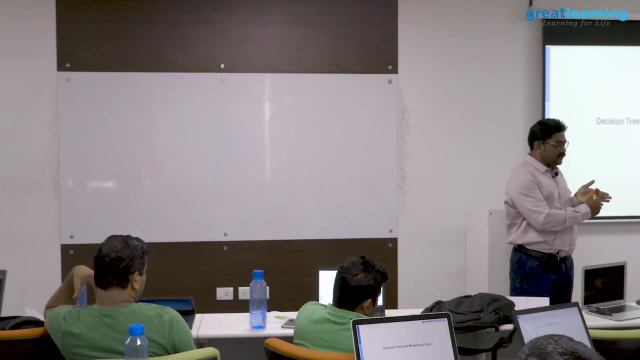 K, Otherwise you will chance of getting tie. 3 this class and 3 this class. your model will pick randomly. Even in case, suppose, if you use 6 neighbors, if the number of neighbors 6, if you mention it, even if tie comes, our model will pick randomly. That is the reason. 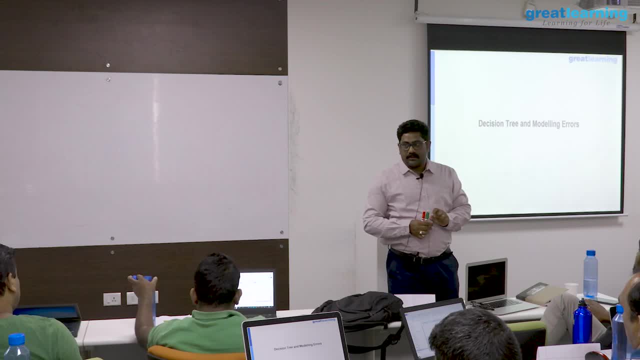 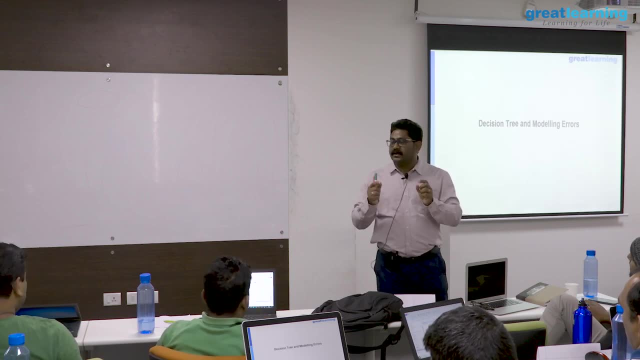 sometimes if you do not set the random state, if you do not set the random state, your results will be different. If you use even numbers for the number of neighbors, every time you run you will get a different score. Slightly your score will be different Because whenever tie happens, 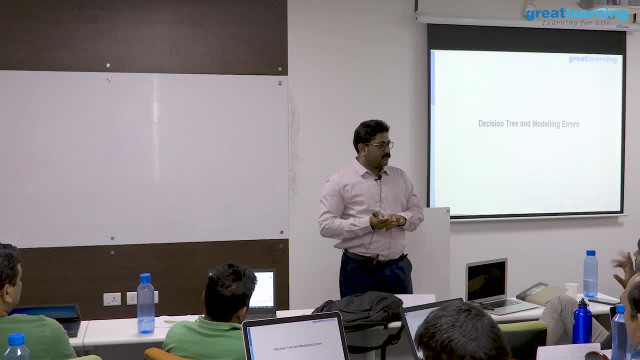 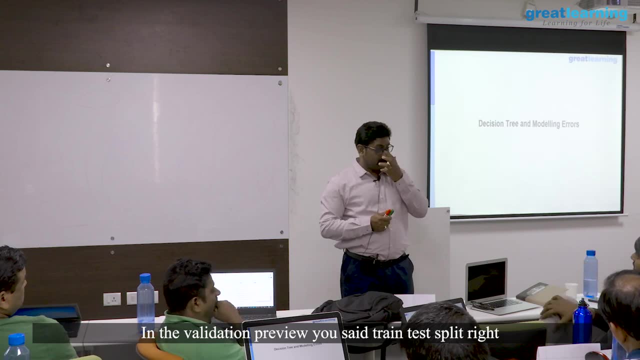 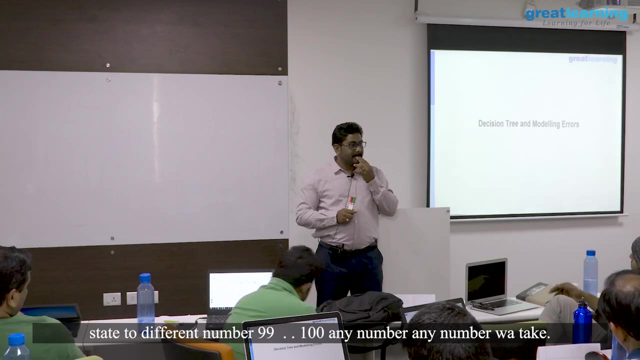 your model will take randomly either 0 or 1.. Yes, I have a question Now. I remember the question: The validation field. you told about the trend test field. There is a field known as random state. While doing the model, we check, we change the random state to different number. We make 9900, any number we make. 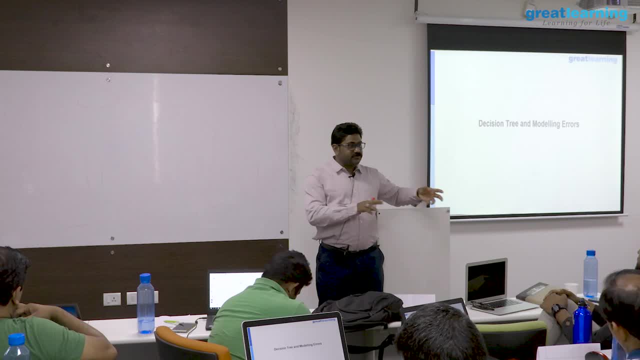 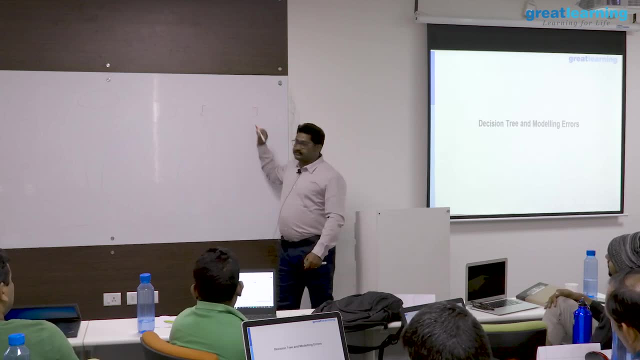 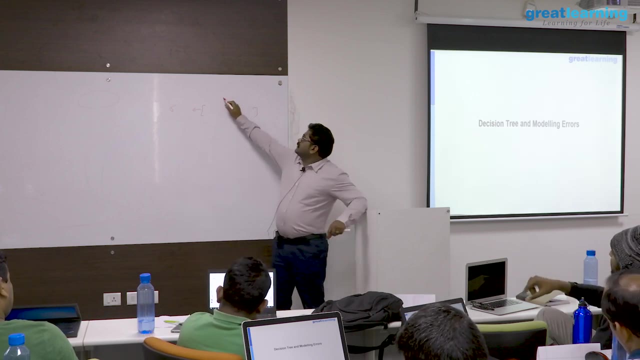 The model, But your range will be maintained the same. Even the individual scores will be different, But it will maintain the same range. How do you check that range? Once you have this range estimate, you have to calculate sigma of this range, standard deviation of this range Range. 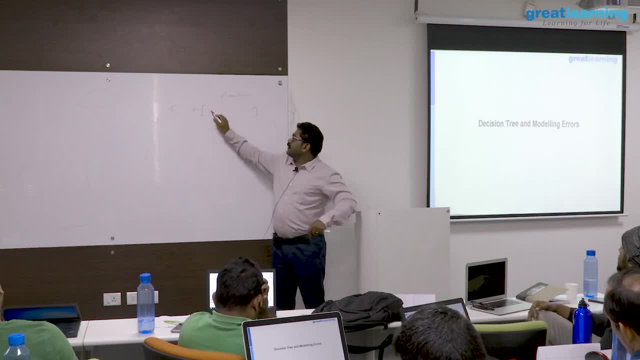 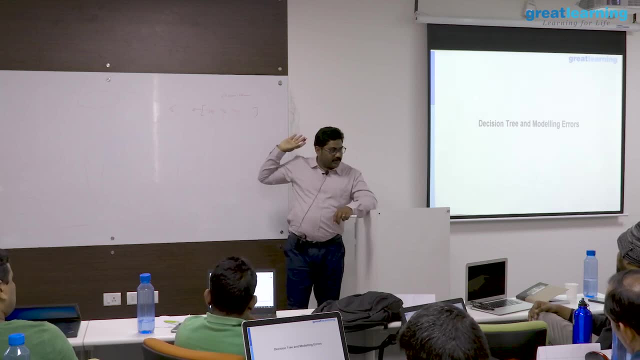 of accuracy score. Accuracy score: This is 78,, 70,, 75 and so on. Different values you get. My individual score can be different, I do not bother about it, But at the end of the day I will calculate. what is the sigma of this? What is the sigma standard deviation? 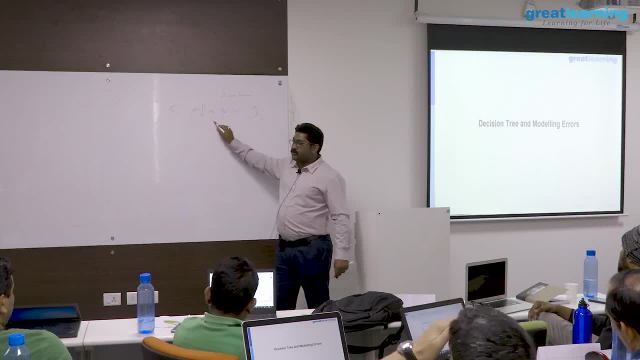 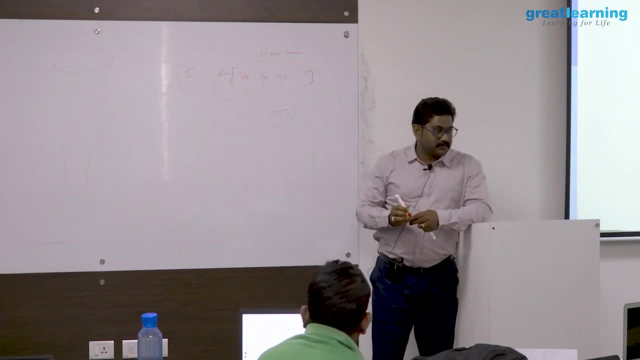 of this percentage is My sigma and average of this. What is the average of this? Finally, I will be reporting this average, and sigma and average should maintain more or less same, Irrespective of which of the record you test. which of the record I test this individual. 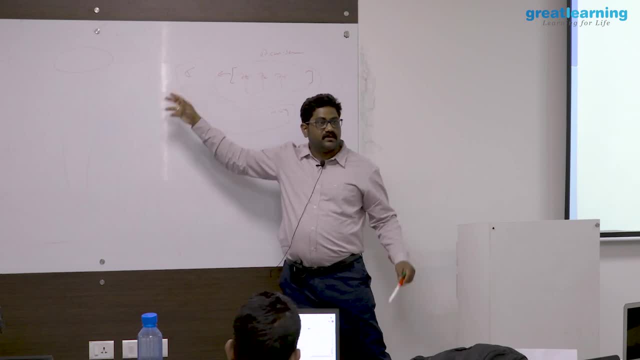 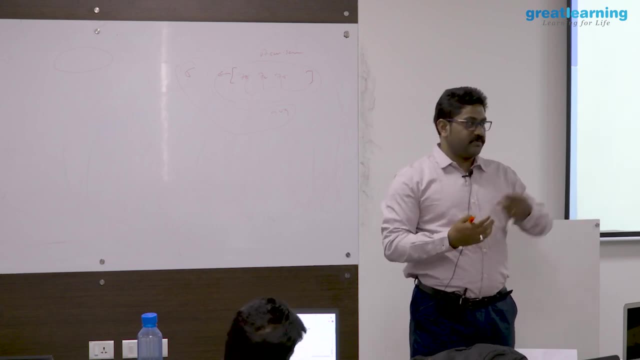 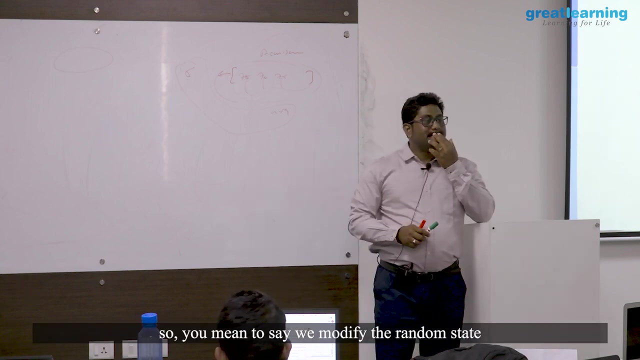 scores can be different. But sigma, What is the sigma Variation in this percentage? right, It is a variation in my percentage. My variation in the percentage is: I will calculate the equal to whatever you tested and whatever I tested, more or less. see why. 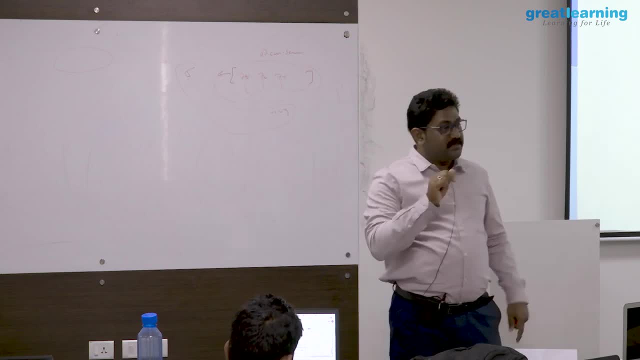 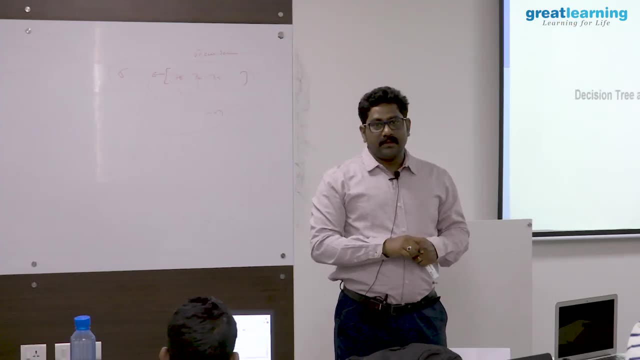 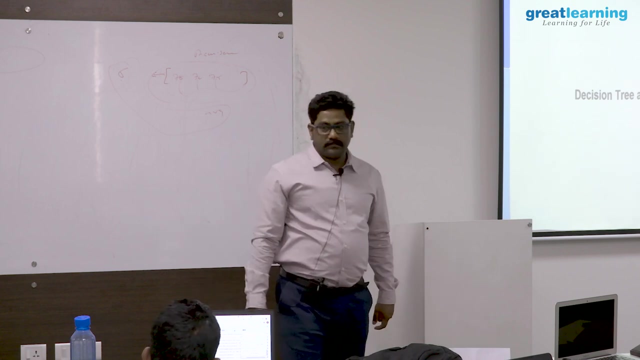 we fix the random one. random state is only for this classroom practice. can you tell me the reason why all of us are getting the same answer but in the reality we don't set random state? because in the reality I want to have the randomness should be maintained, otherwise my model will be biased. the 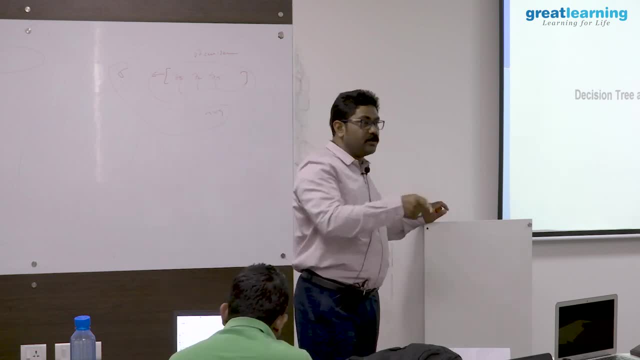 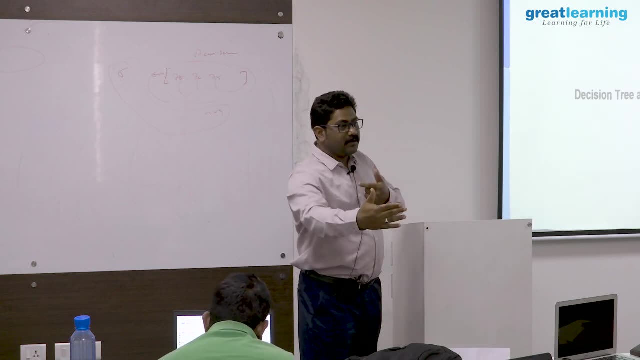 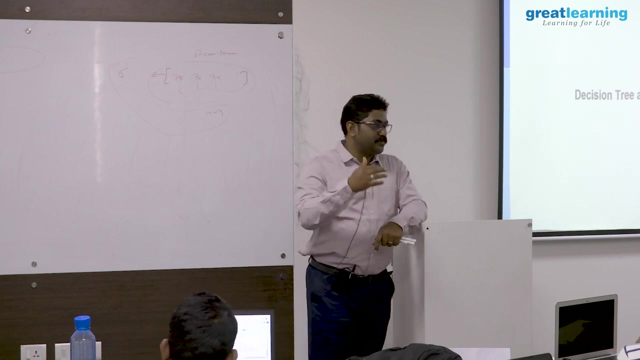 moment you set a random state to your model, you are biasing your model. you are forcing your model to always select this, always. you select this random state is only between my answer and your answers same to cross check only for that purpose. otherwise, in strict sense, and the real production system or in the 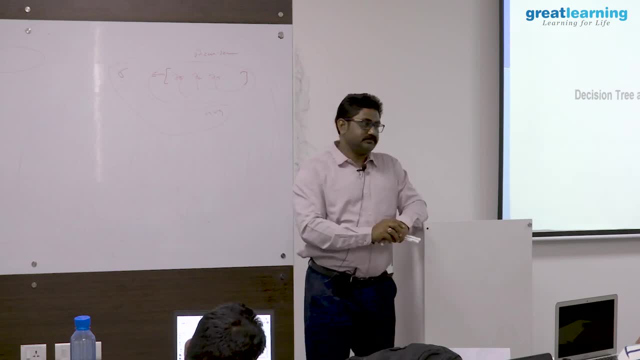 project, whatever you implement, we don't want to have randomness in the reality. we don't want to set random state at all. repeatability, after all it's. you want to maintain the same repeatability even if I do some changes in my hyper parameter. okay, and you want to re-evaluate your model, if at all, if I 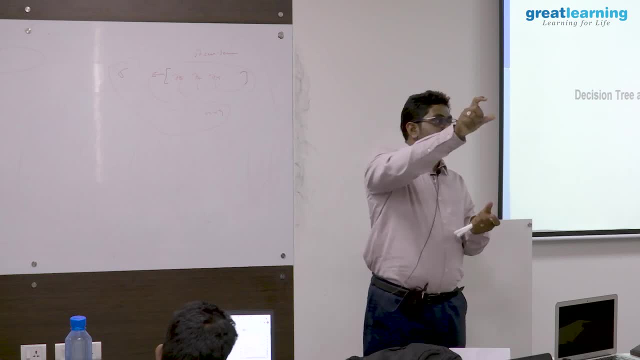 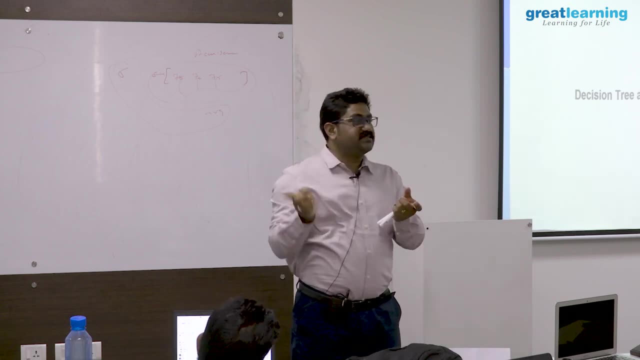 want to pass the same records, then only I can check whether the change in the hyper parameter really makes some sense. otherwise you do some changes: K value from 5 to 7 you change, and this time when you testing it you pass different record for the testing. you are not actually comparing your model performance. 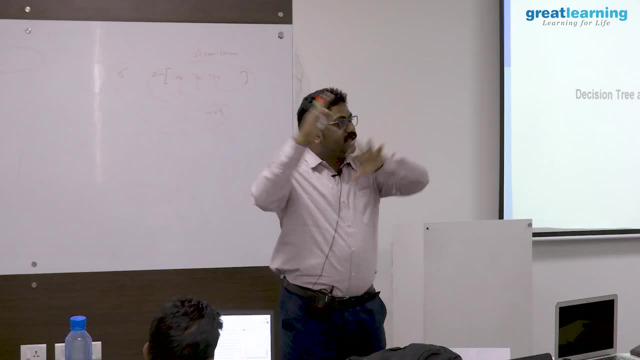 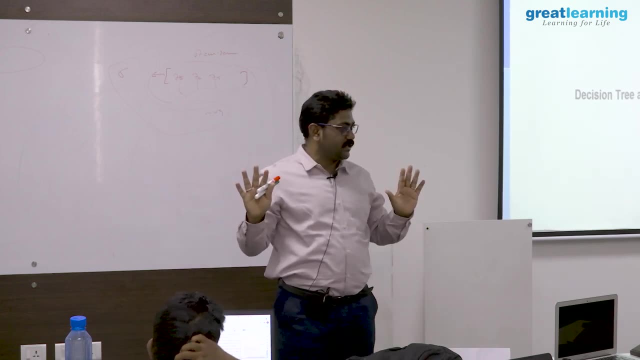 right, because with K equal to 5, you tested at the different records. K equal to 7, you test with the different record. there is no benchmark for the comparison. right, you have to freeze the number of records. these are the records I am going to test for: K equal to 5, K equal to 7, models with the random state, we freeze. 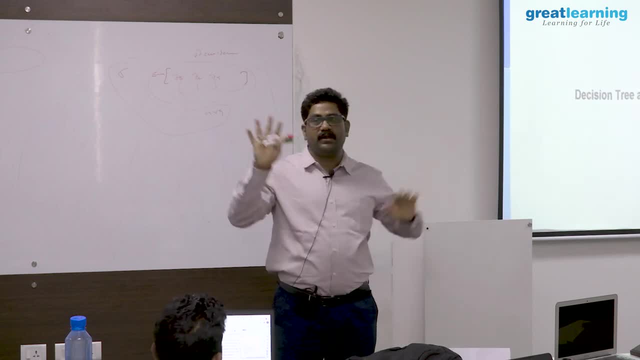 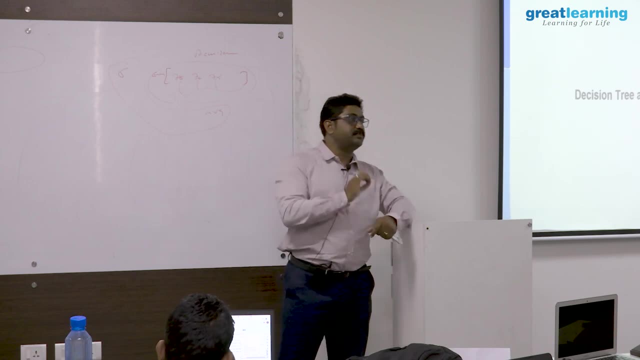 it the same records, then it will make sense: K equal to 5 is performing well or K equal to 7 is performing well. only for that reason, for the repeatability, for the same answer collectively you want to get. only for that purpose, but in the reality 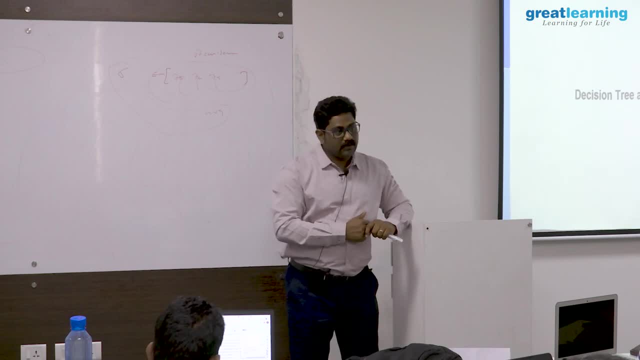 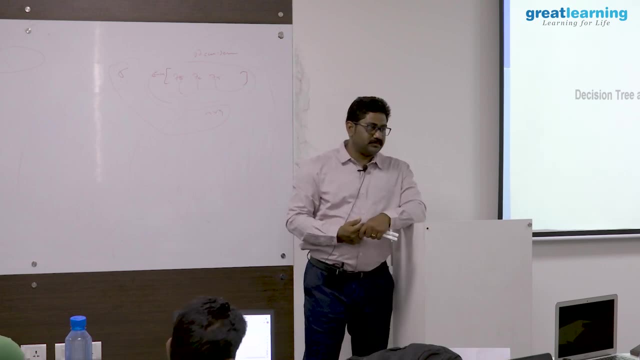 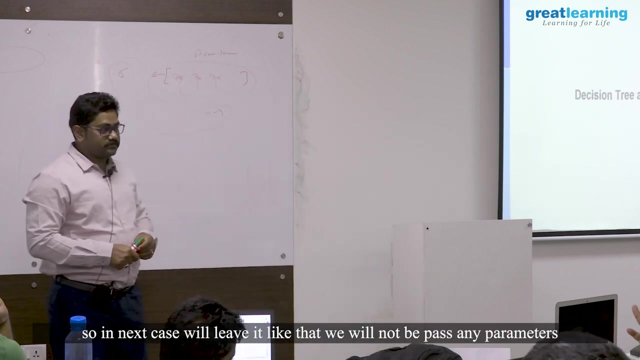 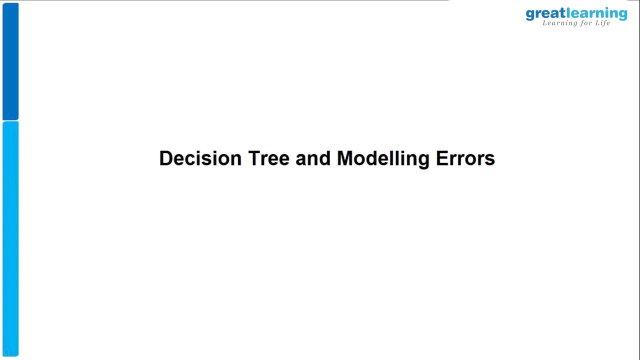 I don't want to maintain the randomness random state. keep it as a real randomness. randomness should be there for a good model, otherwise your model will be like biased model. forcefully you are saying something to choose this. ok, decision tree. the concept of decision tree starts. let us take some example to 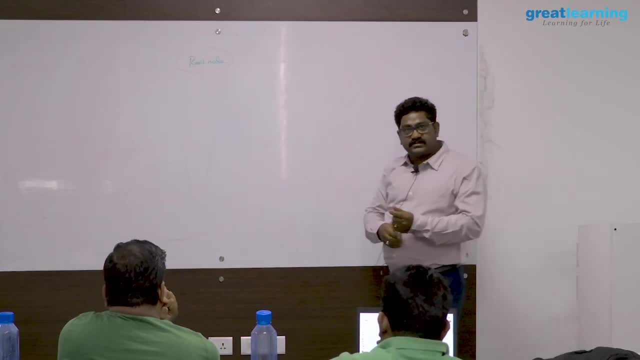 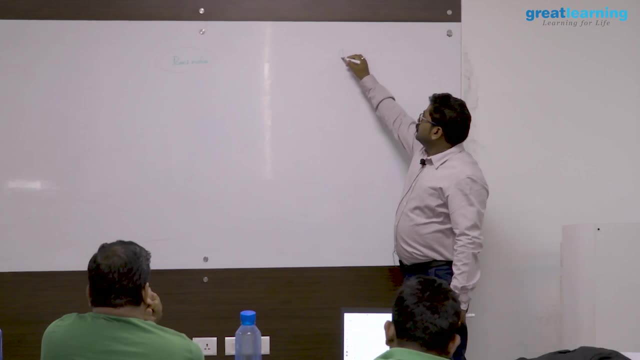 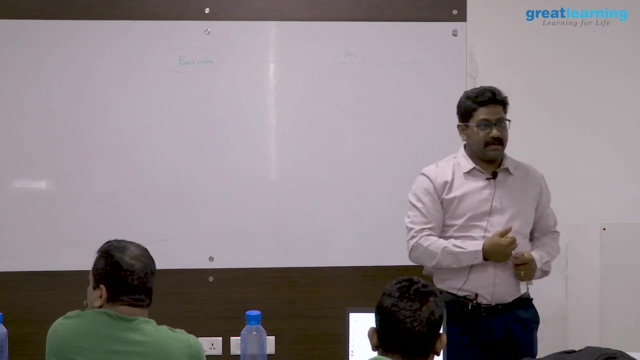 understand this better. first let us appreciate a decision tree as a classifier. as a classifier, then I'll tell you how we can use of it as a regression. also. let us take a some simple example: always any, any model, any model you discuss, or steady, always you. 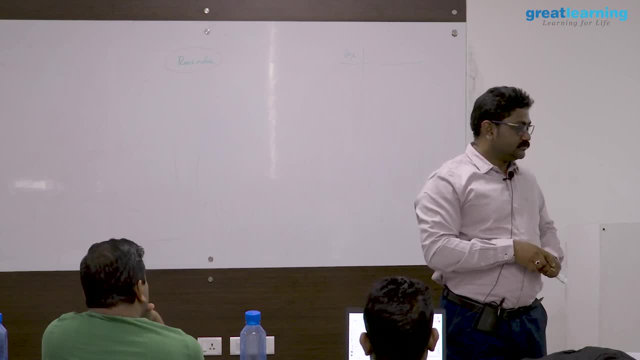 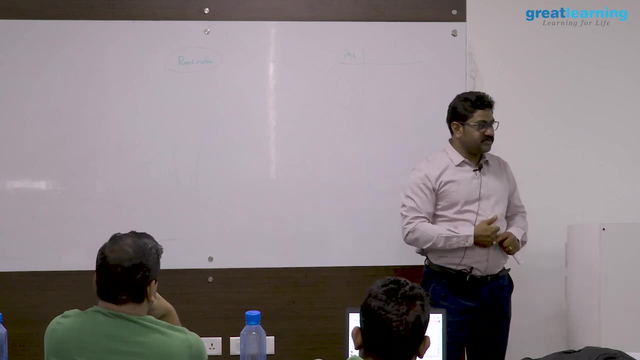 start, apply that model to a some toy data set initially. don't jump into your real data, otherwise it like a black box or opaque. you don't know what's happening at each step will be treating or looking your model like a black box. first you try to apply to this toy data sets what's? 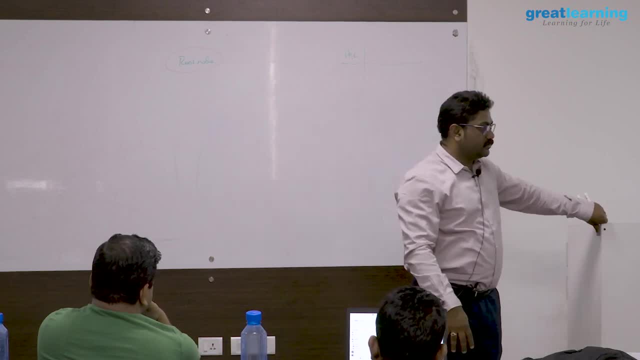 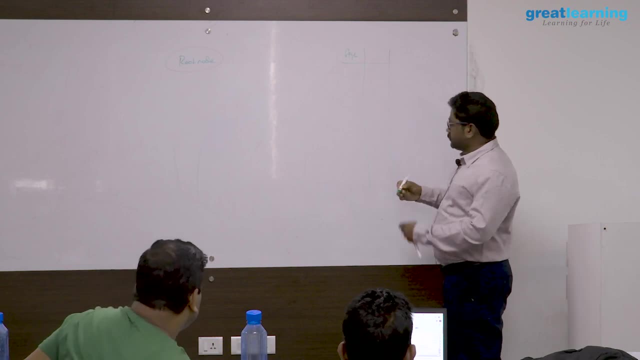 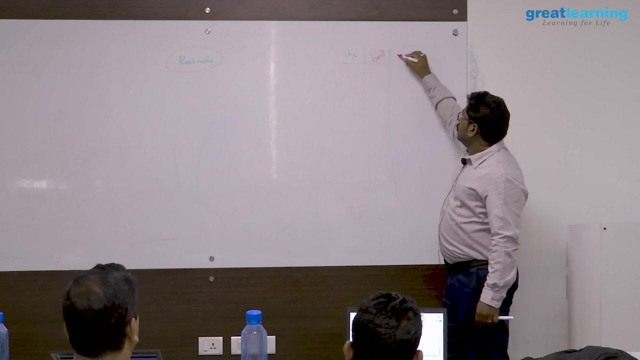 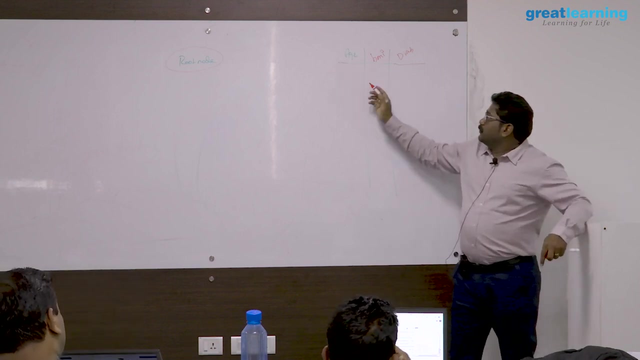 happening. you will get some transparency- okay, this is how it's happening to the data and then you can apply to your real data. so let me have some two parameter like H and BMI. diabetic. it's a classification problem. okay, you tell me roughly because, or it's a everyone will know about common right age and body mass index as 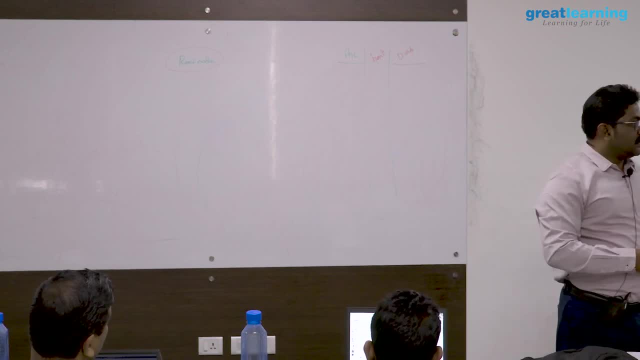 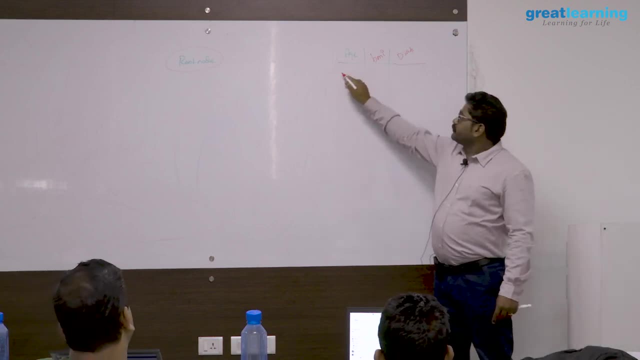 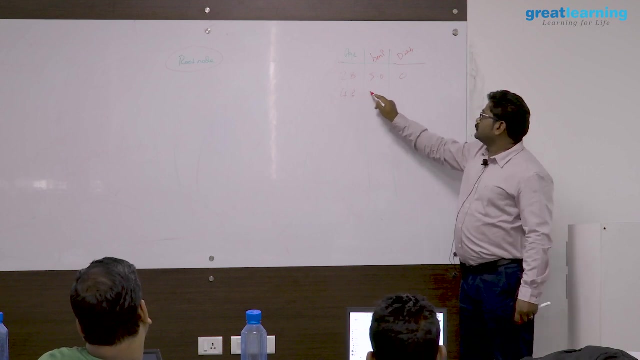 BMI increases, we have high risk for the diabetes obese person. as you are highly obese, you have a high risk of diabetes. you just give some some pair of data: 28- 5- no diabetic. 48, 7.3. I keep it. 134.8 0. 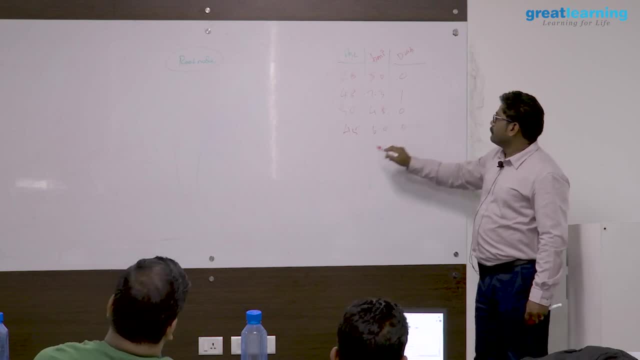 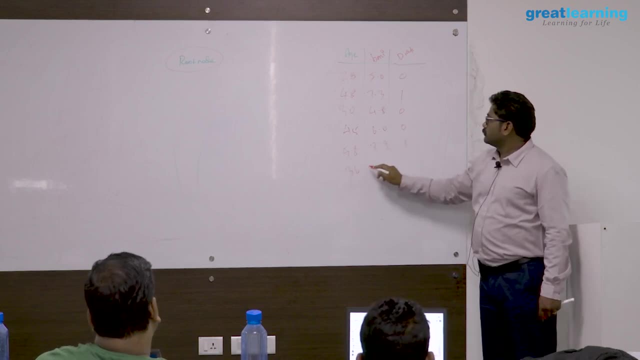 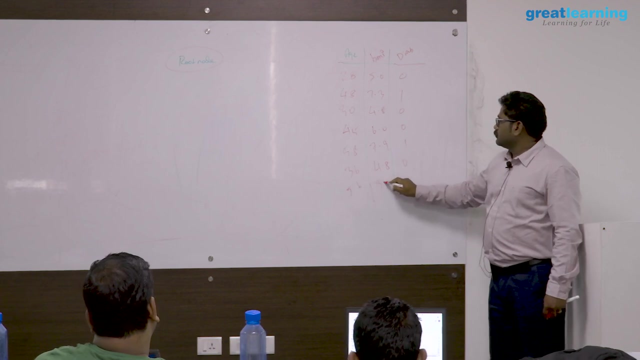 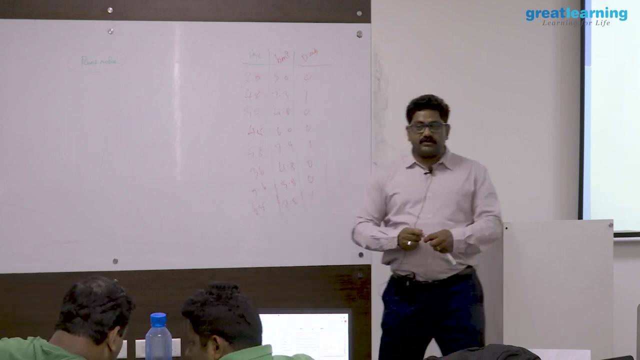 ok, let us assume this is my, our data set. 5, before you go to the other side, as you can tell, let us assume if you have two models like molecular network versus fluid model, because let me make it cheese if you have one spicy Oreo course, let us assume they stick on each side so that one is resistance. 1. Shore בש and Boulogesh. 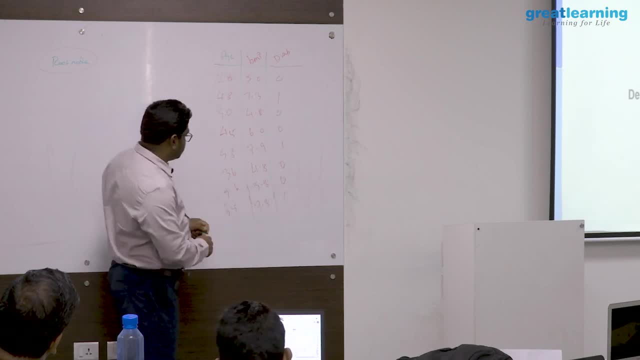 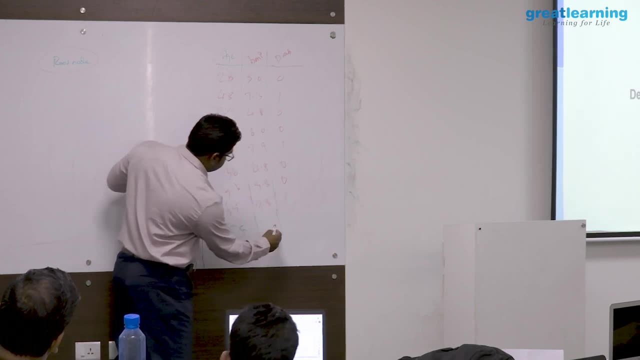 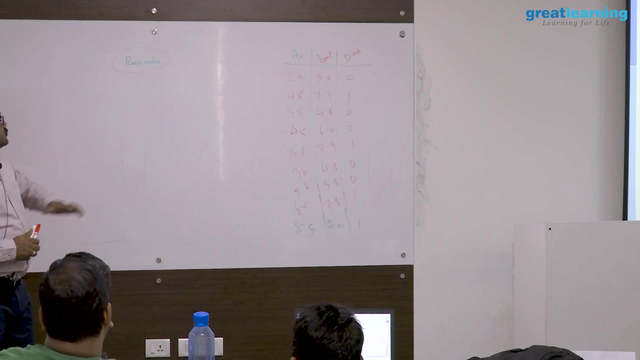 Let's not forget using a vector molecule. ok, let us assume this is my. our data set: one, two, 334, 5 from two, three diabetic cases. ok, let me take one more. So we call: we start with the root nodes decision tree. we start with the root node in root node. 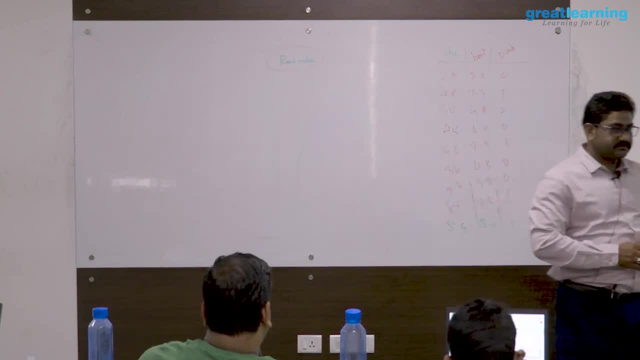 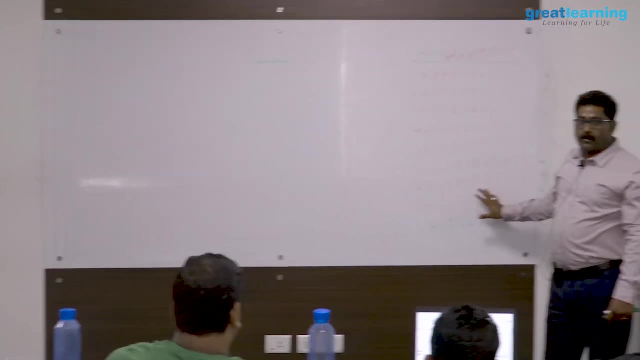 my entire records. I am going to consider, as my training samples assume, I am going to build my tree. I am going to build my decision tree with my training samples. this is my training samples. how many records? I have 9 records, right, totally, we have 9 records, all the records. 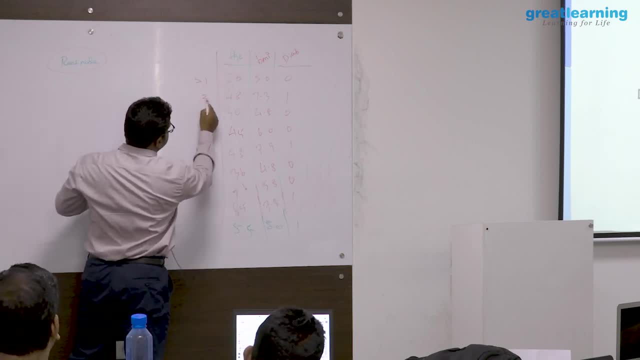 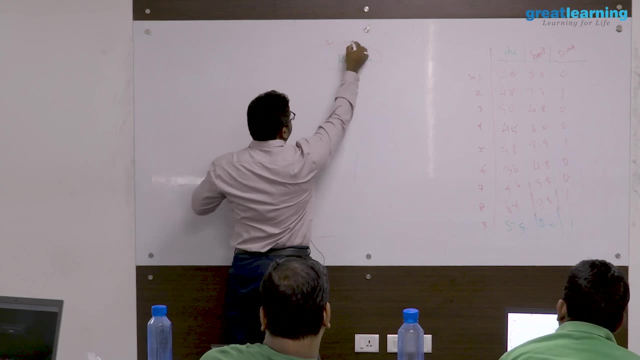 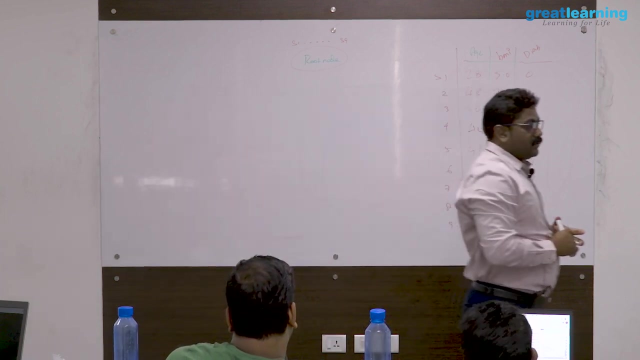 are I listed out here? so let me say record numbers: sample: 1, 2, 3, 4, 5, 6, 7, 8, 9 at the root node S1 to S9. all my records are here. So here I am going to introduce the two terms here, irrespective of your discipline, engineering. 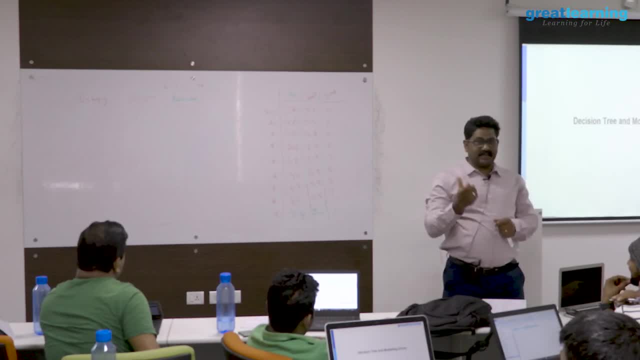 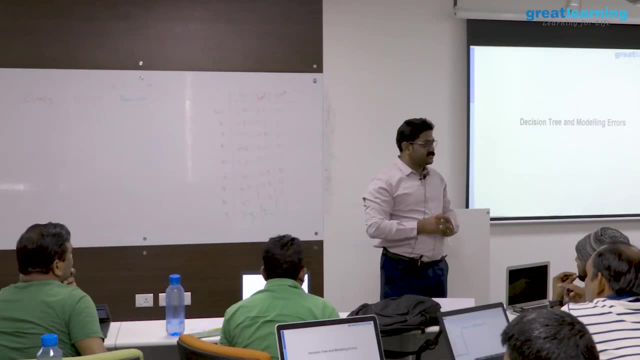 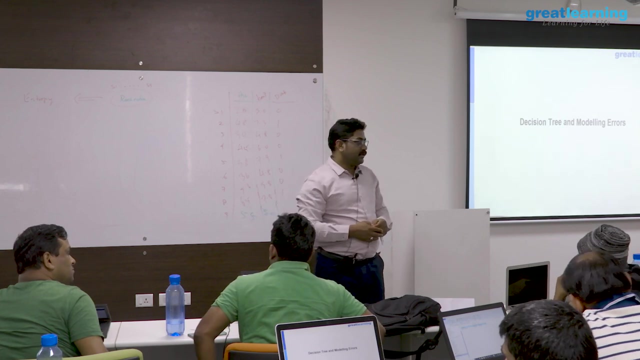 discipline. definitely, we come across this. basically this, actually this entropy is a came from the communication engineering, information theory Shannon, proposed by Shannon scientist, Shannon entropy. entropy is a measure of randomness. also you can call it as a measure of uncertainty. what you mean by uncertainty, for example, at the root level node? assume that at the root. 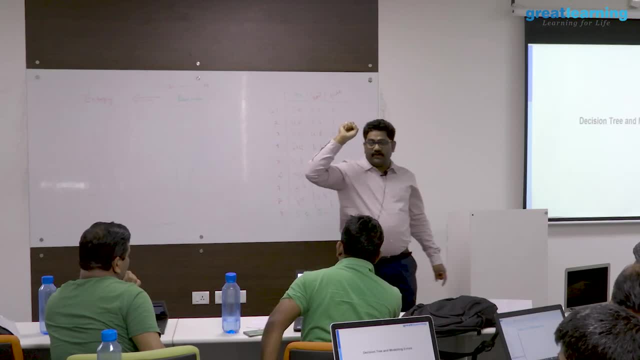 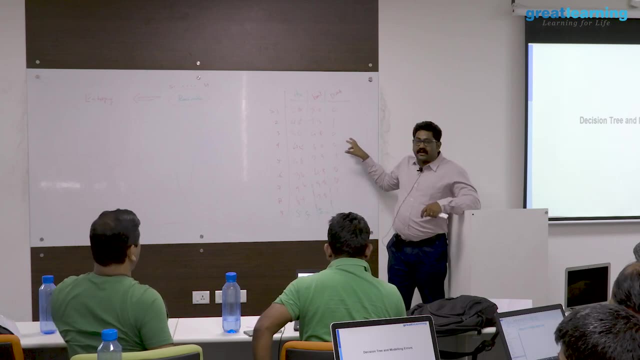 level node randomly. You are going to pick one record And you have to say whether it belongs to class 0 or class 1. what is the chance? what is the chance of getting 0 class 0 randomly? or picking one record and you want to say: 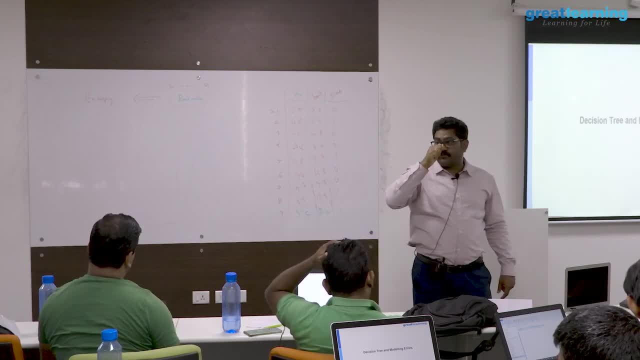 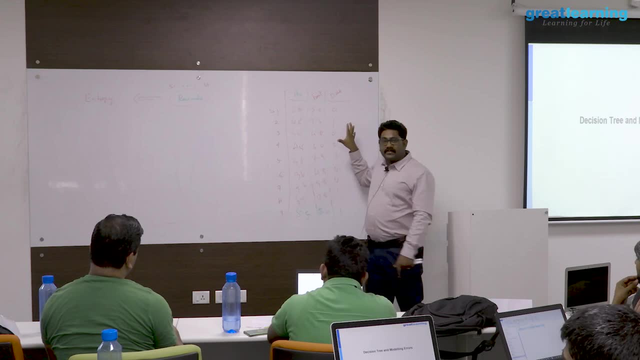 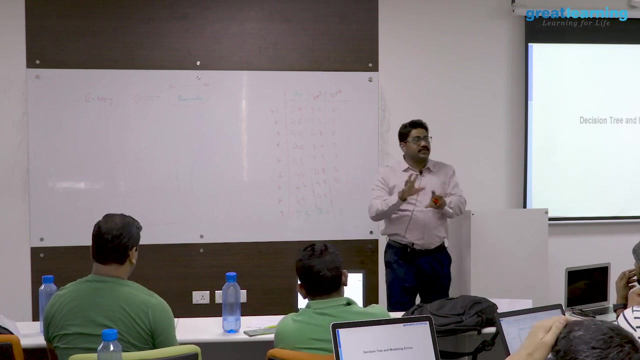 diabetic or healthy? what is the chance of what we call in other way? I can call it as a prior probability, right? what is prior probability from the given data set, from the given data set, from the historical data? it is a known probability. you do some transformations on. 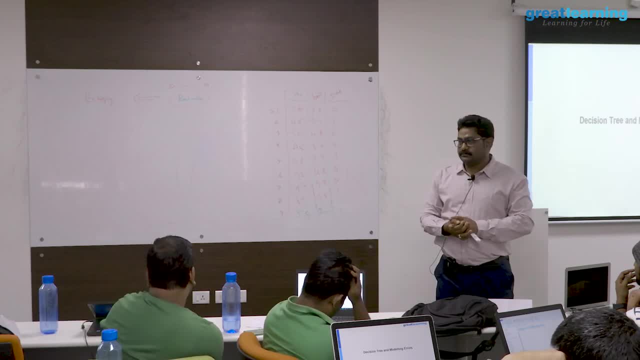 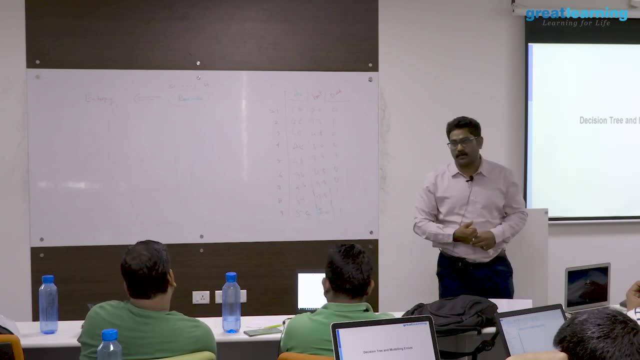 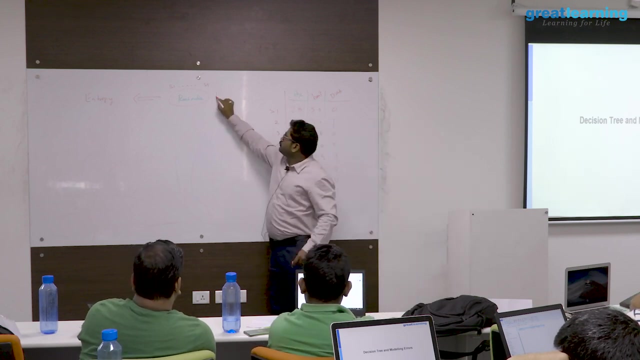 the data and then you calculate probability. it becomes posterior probability. one is prior probability before you process the data. after processing you calculate your probability. it called as a posterior probability. that is prior probability and posterior probability. now, what is my prior probability of? what is the probability of class 0? how do you calculate? 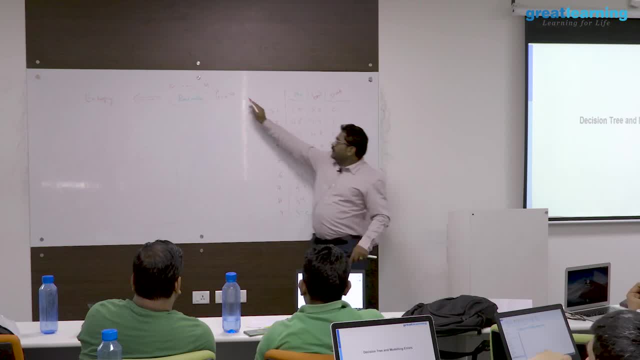 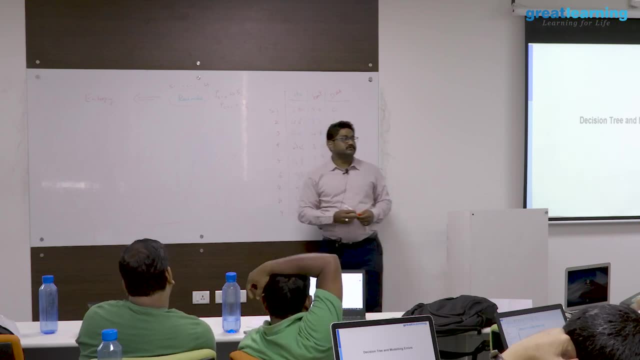 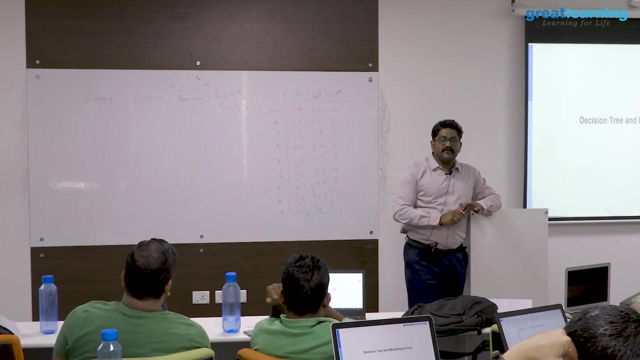 what is the? how many records? 5 records out of 9? 5 by 9 is a probability. what is the probability for class 1 record 4 by 9.. Ok, if it is 5, 0, 5, 1, it will 50, 50 right, 50 percentage, 50, 50 chances, which is the 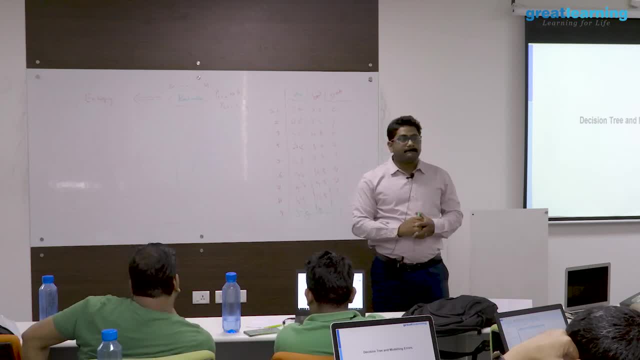 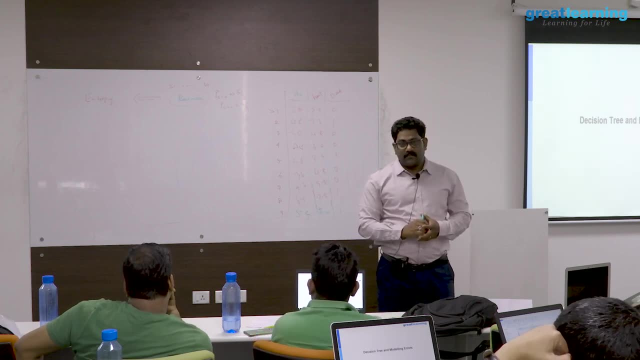 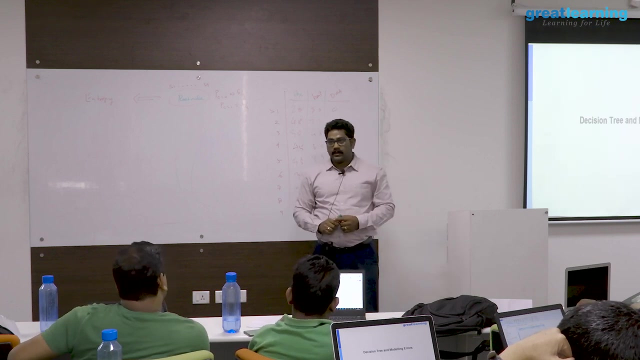 highest level of randomness. highest level of randomness when entropy is 1, we call it as the highest level of randomness. when you will get entropy level 1, you get 50, 50 probability. if I get 50, 50 probability, let us say probability of class 0, but here it is not exactly 50, 50. okay, assume that if it. 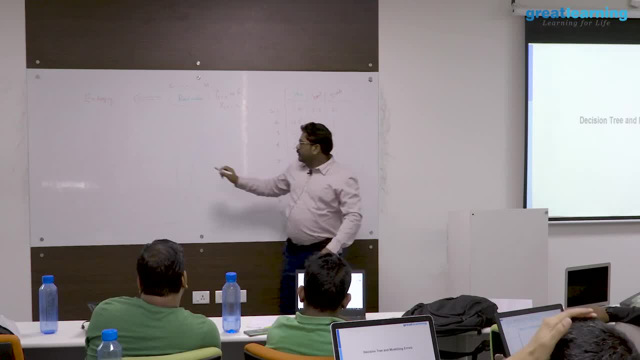 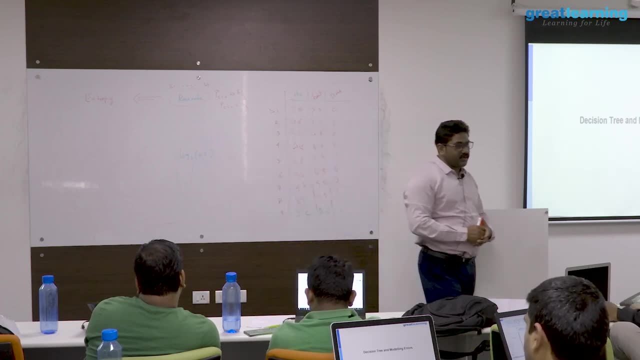 is 0.5, 0.5, 0.5, 0.5. calculate log base 2- 0.5 and tell me quickly, use any tool and tell me you can check it in Google. what is log base 2, 0.5. 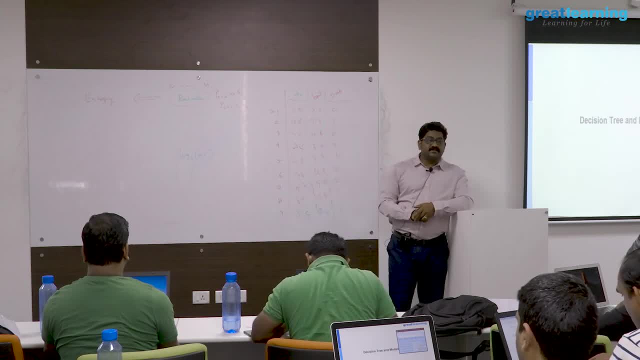 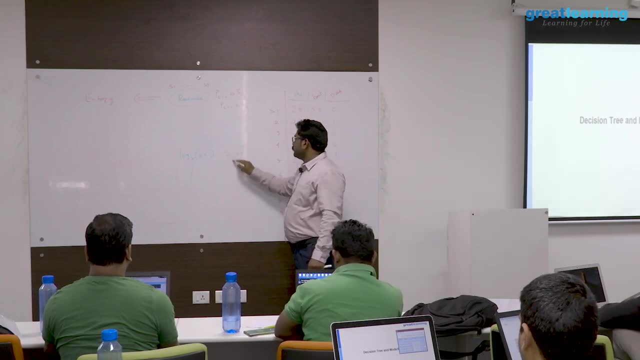 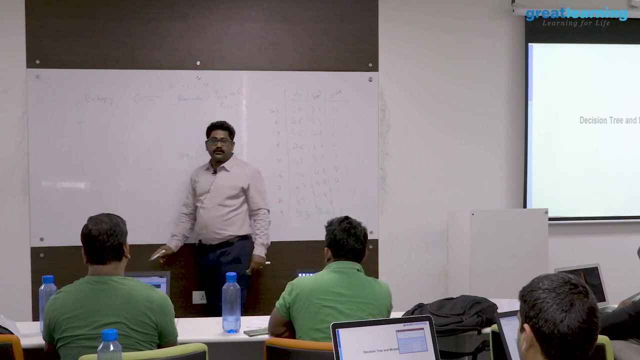 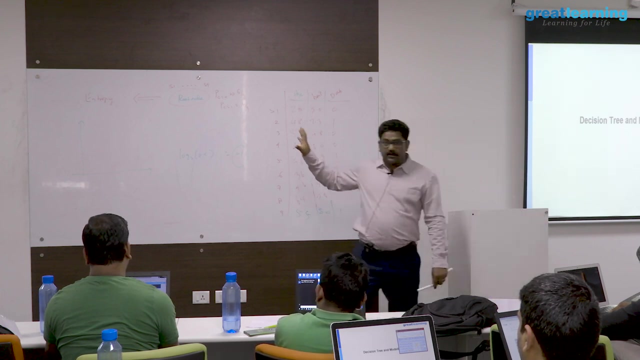 log base 2- 0.5. your base is very important. we have log base 10 natural log and log base 2 minus one. we are going to have relationship, what Shannon has framed. the two scientists formulated the measure of uncertainty. this is we are going to. 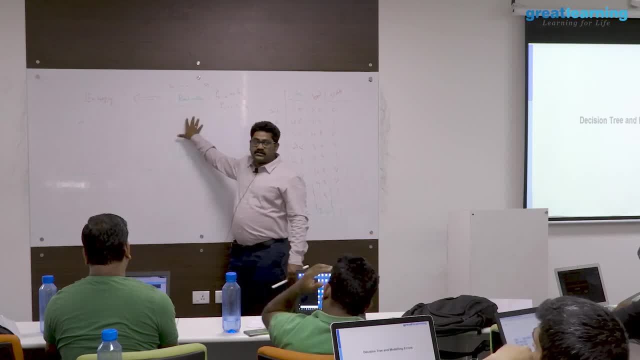 calculate the measure of uncertainty. one is Shannon. another person is a social scientist who worked on the ecology based projects. you can see that this is the measure of uncertainty. this is the measure of uncertainty. you can see that this is the measure of uncertainty. this is the measure of uncertainty. 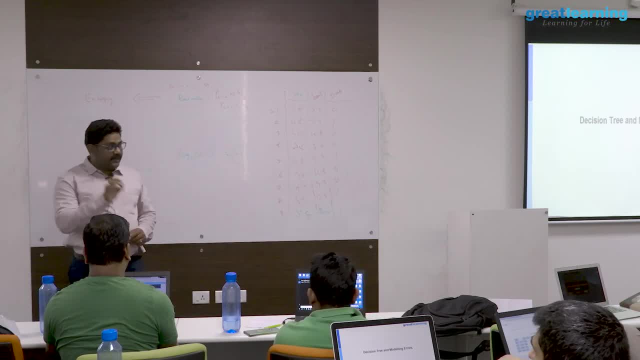 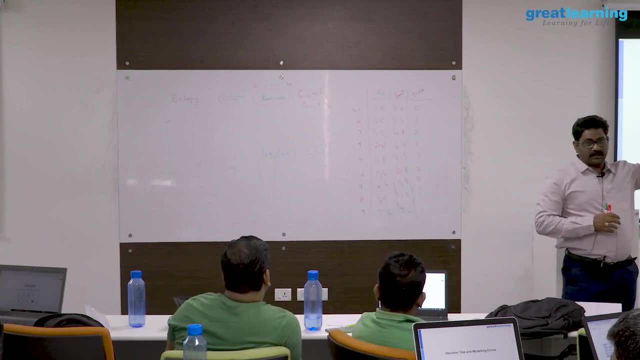 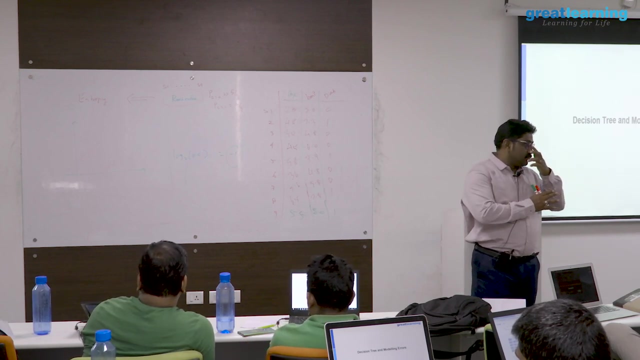 he formulated Guinea index. guinea index also. it's a measure of uncertainty, but both both happens parallel a without knowing that one more parameter is there. either you can go use guinea index as a entropy measure or you can use entropy. both has same meaning. okay, first let us explore entropy, then I'll. 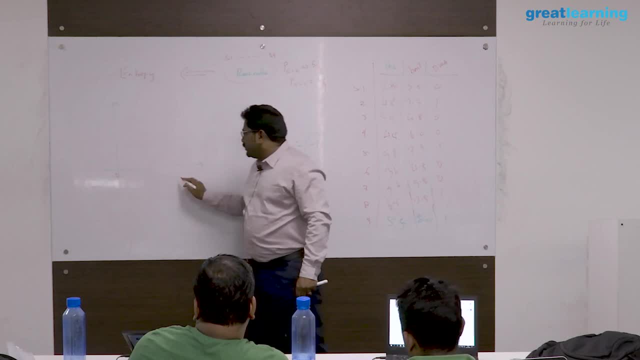 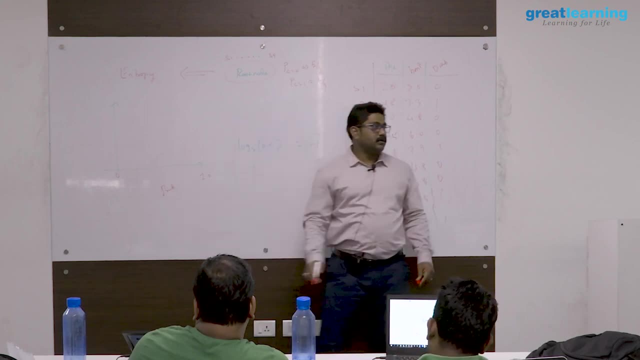 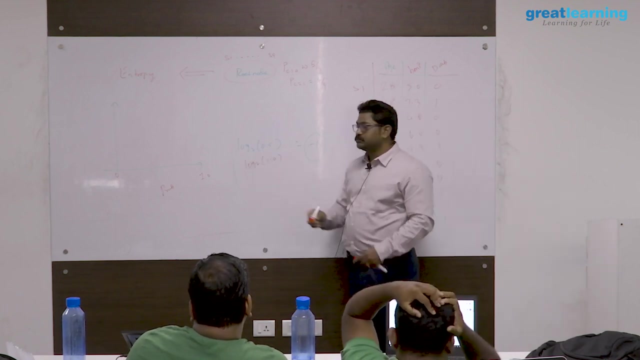 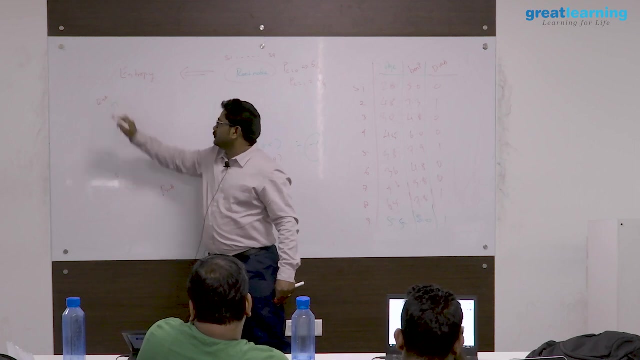 come to guinea index. so what is the maximum probability? the x-axis? I am going to take probability, 0 probability, and this is a maximum probability: 1. what is log base 2, 1? sorry, log log base 2, 1 is log 1: 0. so when probability is 1, your entropy y-axis is entropy. entropy is 0. 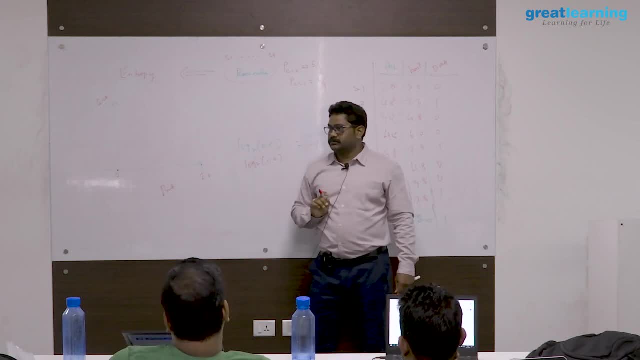 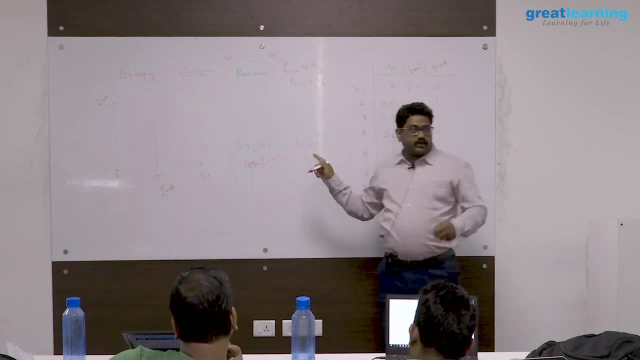 okay, when probability is 1, my entropy is 0, 0 comma 0, point right. and this is at 0.5. at 0.5, how much you got minus 1? for time being, you ignore this minus 1. I'll come to this minus sign shortly. my entropy is a maximum entropy. this is 1. 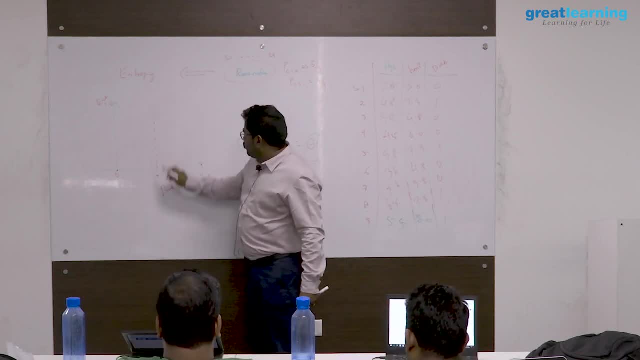 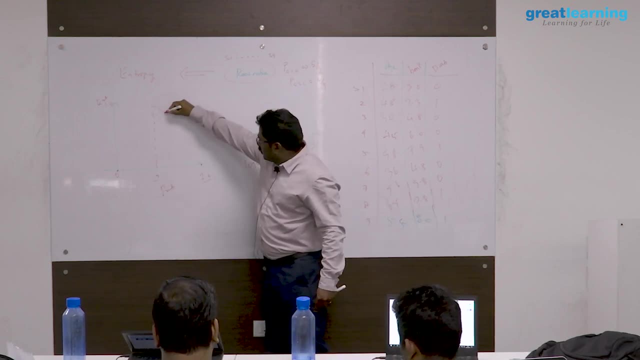 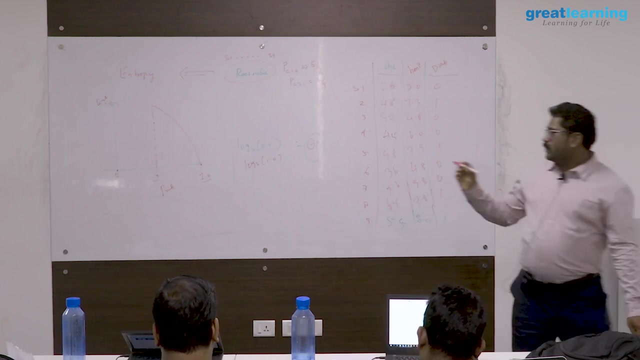 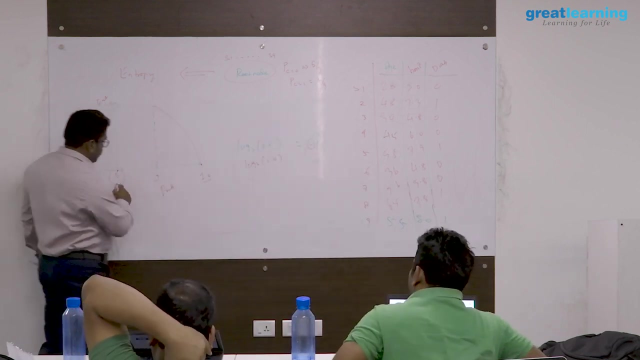 okay, in between 0.5 and 1. if you calculate for any other value- 0.6, 0.7- and if you connect the points, it will come like this: calculated, you can see the score and you can connect it. this is a way. your values typically. what is probability at 0 log base: 2: 0 log 0. 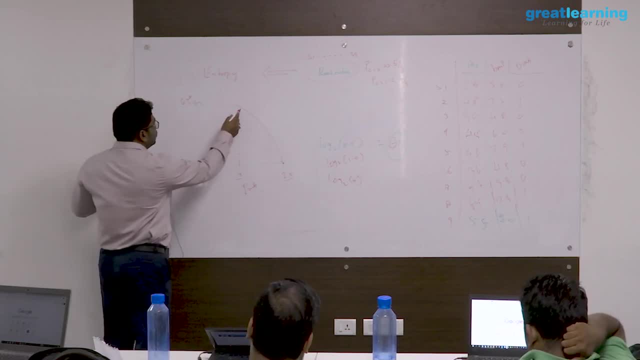 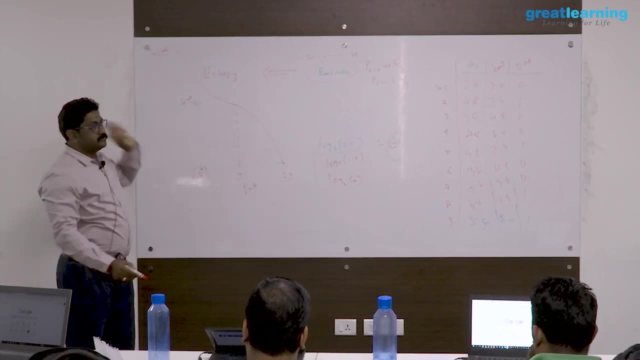 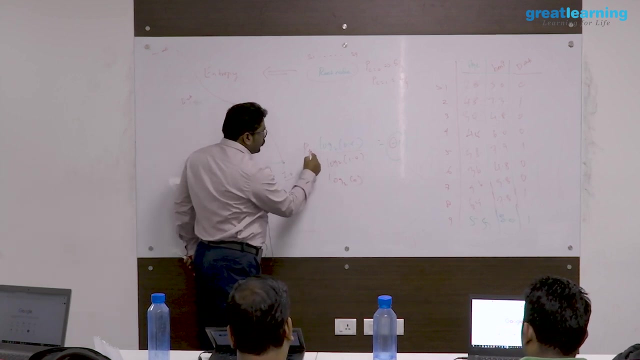 minus infinity. minus infinity, that means strictly, if I use this equation. what happens? Shannon observed, your entropy goes like this: minus infinity. so what he did is he multiply with that probability score P I into log base 2, P II. that is a formula. what is the entropy formula? 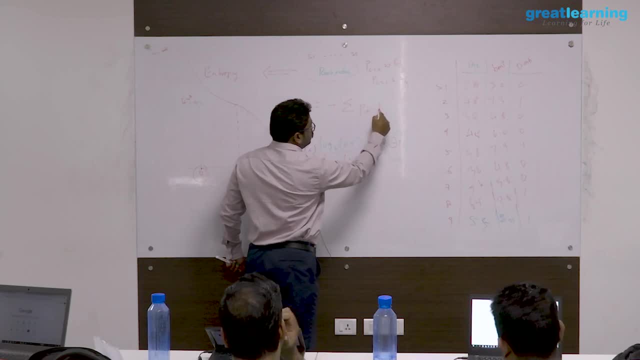 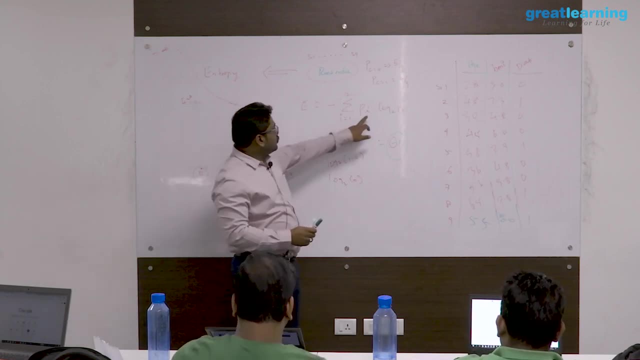 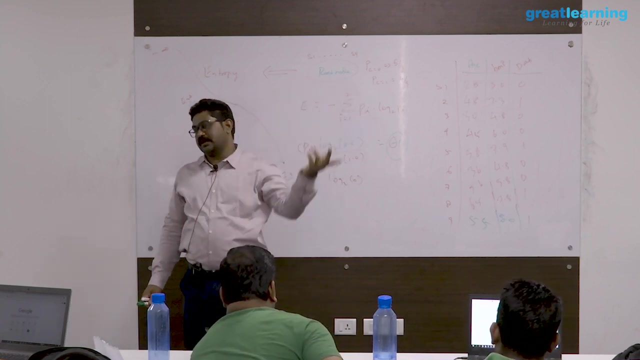 minus. summation of P I into log base 2. P I- what is I is one to two. number of class. when I is 1, what is a probability the of your data belongs to first class? when I use two, what is a probability that your data belongs to second class? 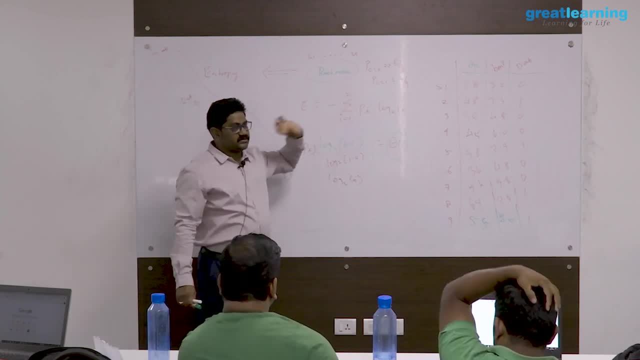 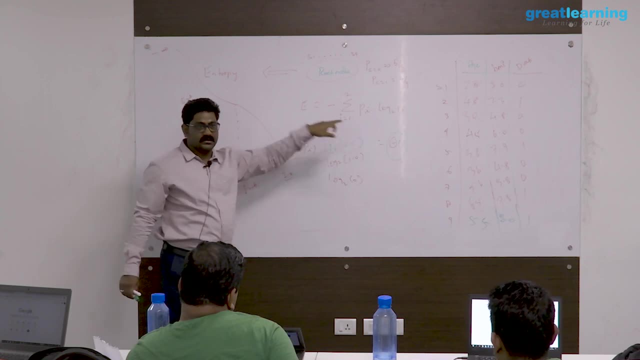 we can call it as a 0 to 1 or 1 and 2, whatever, it is just a label. okay. PI into log base, 2 P why he introduces minus sign to negate the minus effect. minus into minus 1. it become plus 1, right, so my entropy level will be plus. 1 is the highest level of. 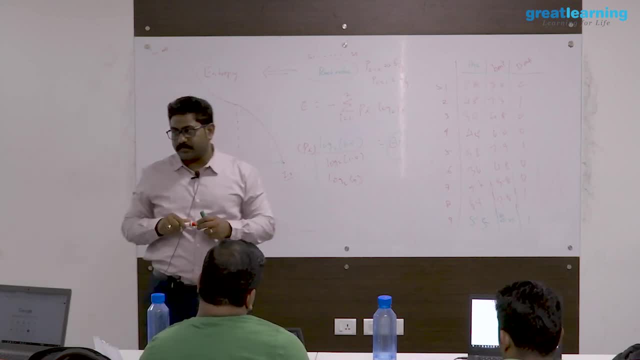 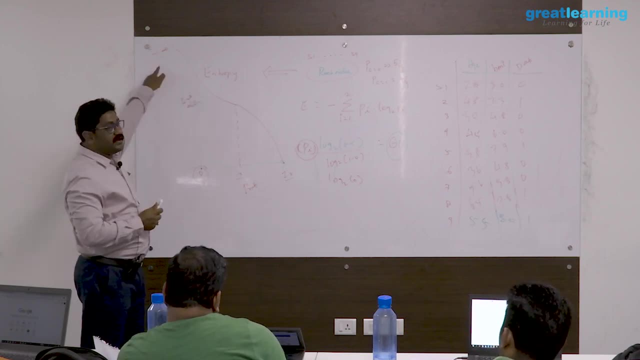 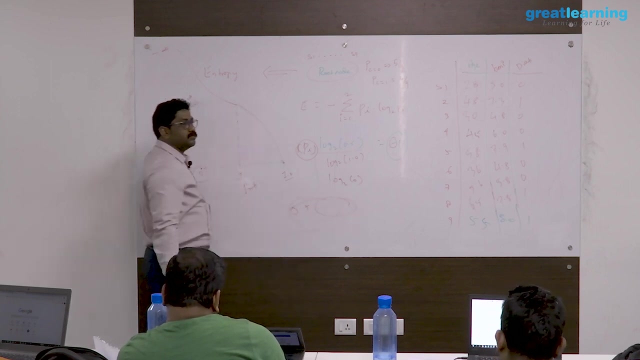 entropy, if entropy 1 means highest level of uncertainty. so when you multiply with this probability, for which value of P I, you got minus infinity. log of 0, you got minus infinity. irrespective of whatever the big number you multiply with 0, entire value becomes 0, right? so between this value and 0.5, you are the trend of. 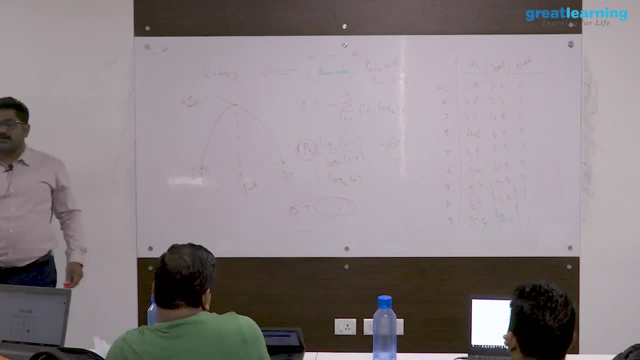 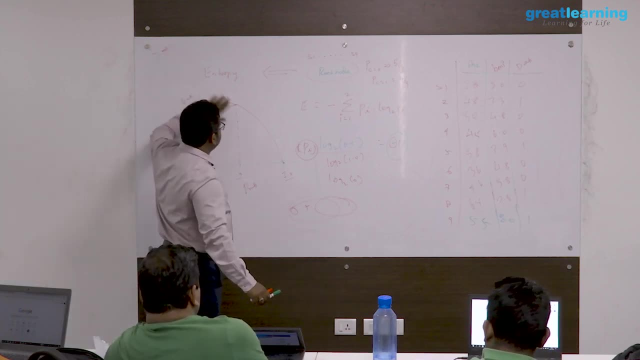 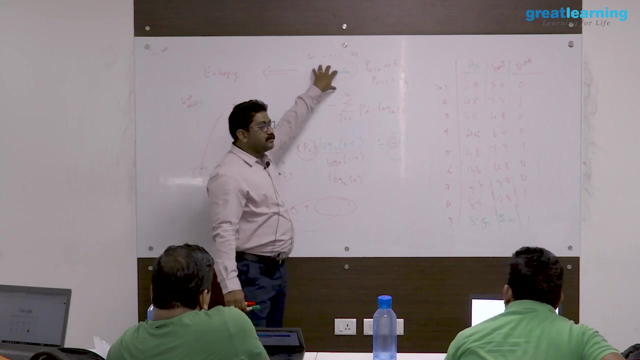 entropy goes like this: this is how Shannon formulated the relationship between the probability and entropy. so this is a relationship of probability and entropy and the corresponding equation is: this is the equation- what decision tree is going to do? it is going to measure the entropy level at the 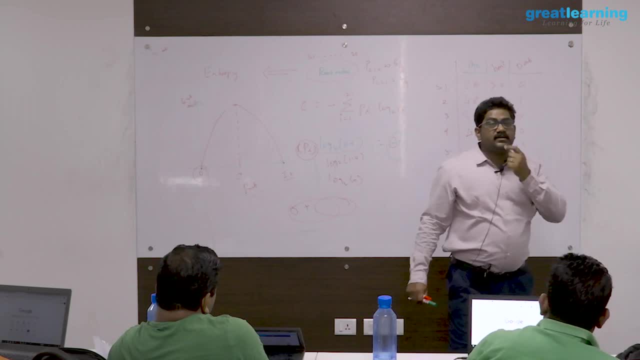 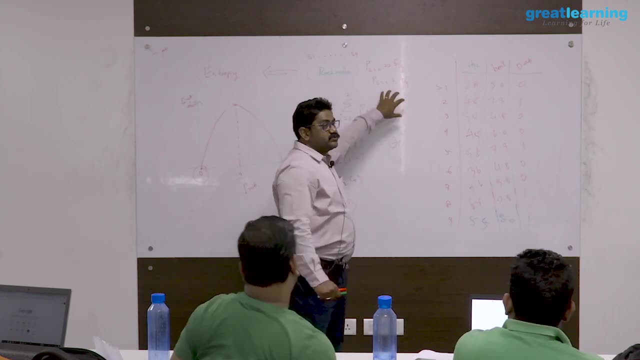 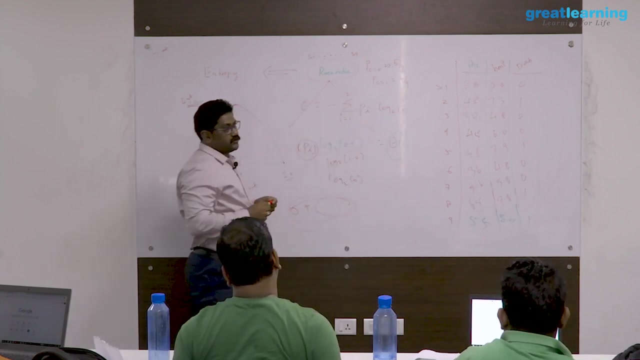 given data set training samples. my entropy level is very high in the sense what there is a high level of uncertainty. deciding which is like class 0, which is class 1, is very tough here. that means you are going to branch out. here your decision tree is going to make a branch out. 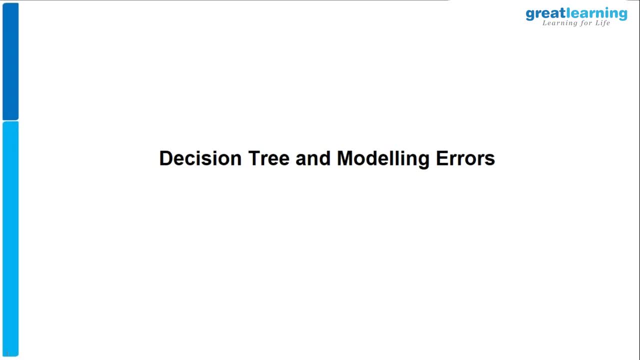 what is log base 2 of 0 minus infinity? but as per the formula, we have to multiply the probability value. the 0 is nothing but probability P I. so I'm going to multiply P I into log base 2, P I 0 into this any. whatever the big number, it becomes 0. so that is why this: 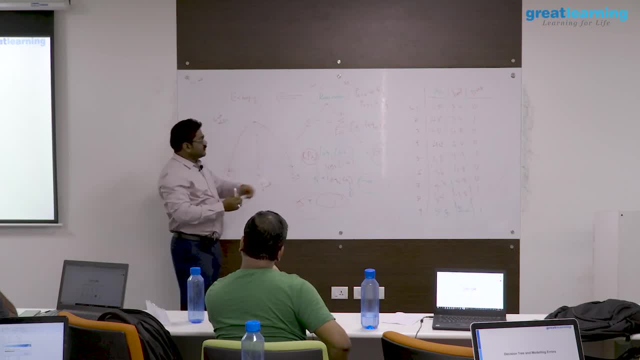 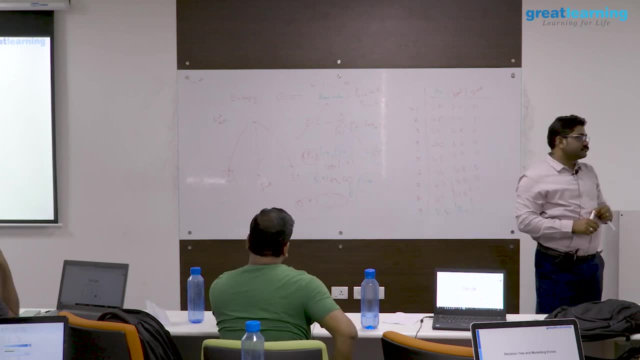 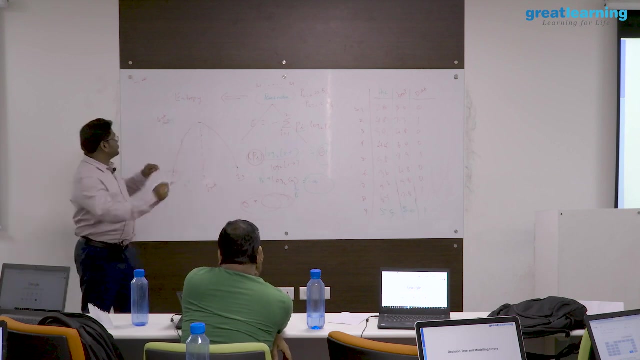 graph will be controlled like this because of this multiplication factor P I, it will be controlled from 0.5, sorry, 1. again it will be dropping any value substitute between, for example, 0.3. you just substitute and check. you just check for example 0.3 into log base 2: 0.3, again you get negative value. 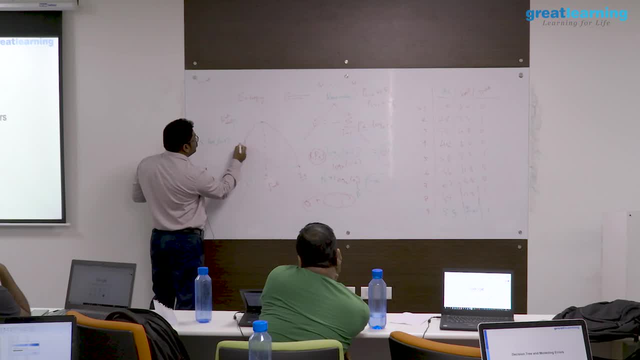 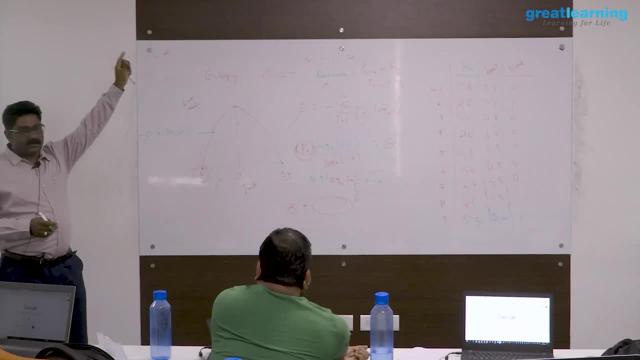 because you multiply with minus, become positive for 0.3, you will get some values close to 0.6 or 0.55. it will not go towards infinity because of this scaling factor P, I, we are multiplying and minus sign you can cross check how much it. 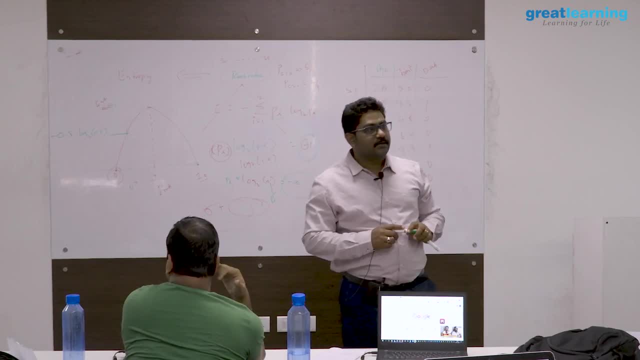 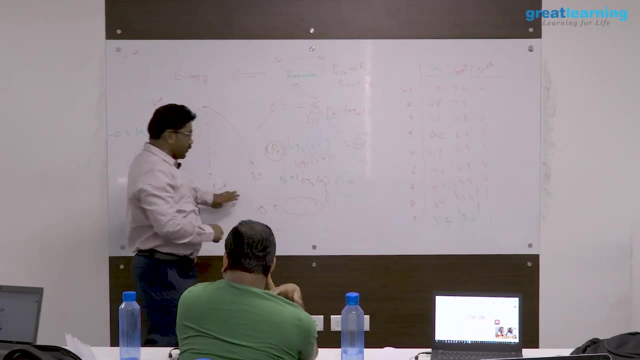 comes 0.3 into log base 2, 0.3. here you have minus sign P. I is 1 plus nigu, or to add. does that sure you have enough to go back to the reference 2 to 0?? yes, how do you do that measure the MY plus 0? so the important thing, 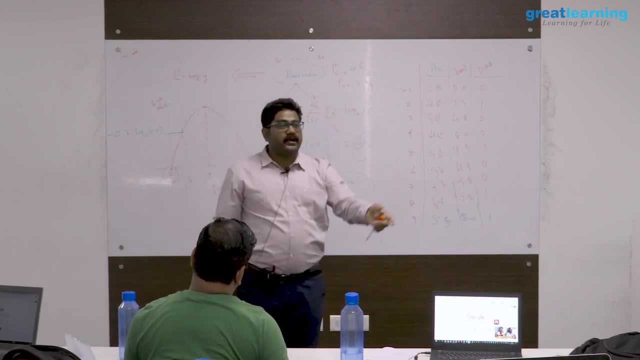 to do is to have the期 Flann guy, the FIFL which I have, I am an names and I am just going to press ok. the�면 y, y axis is the entropy 0 to 1. this axis is probability. this is probability and entropy, because our entropy formula, entropy depends on the 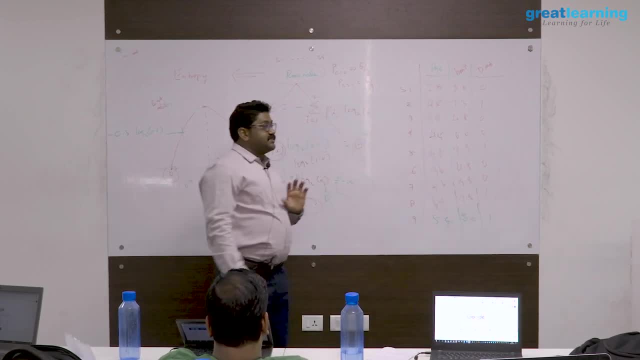 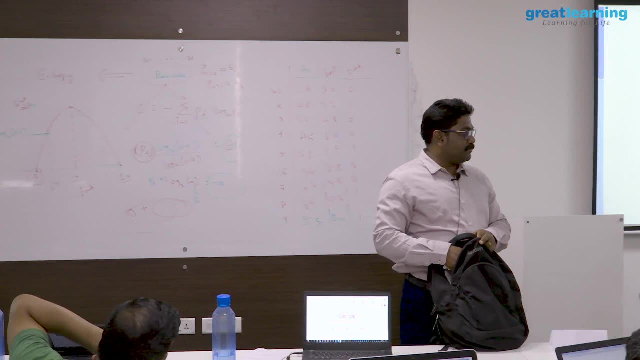 probability rate 0 to 1. now that you remember the Ye email, what is a property that your record belongs to? a particular class, 53 professionals. imagine I have a black bag. listen, i have this closed back. I kept some five red balls and fight black 못. 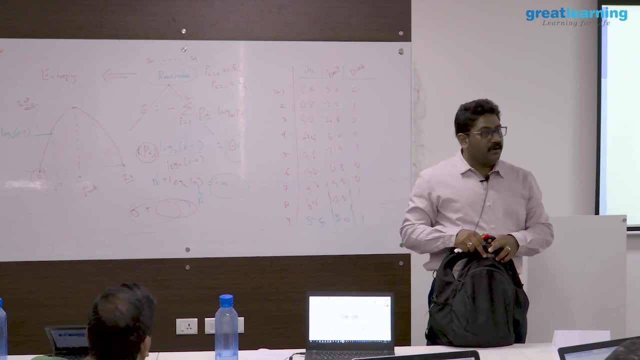 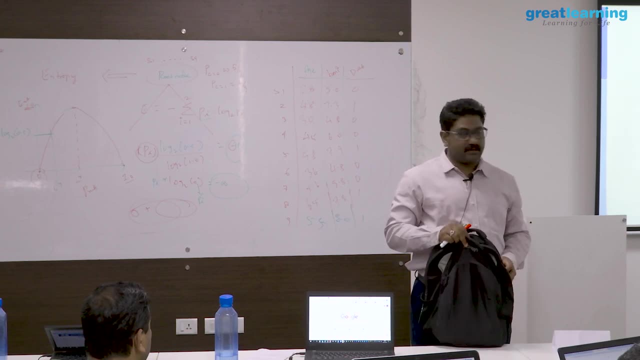 okay, I shuffled it. you reliable? you are the answer: yeah, so the there is 1 normal cannot be collected from эта. I'm asking someone to take one. the chance of getting a red ball and chance of getting a black ball is 50-50 chance. the level of uncertainty is very high. 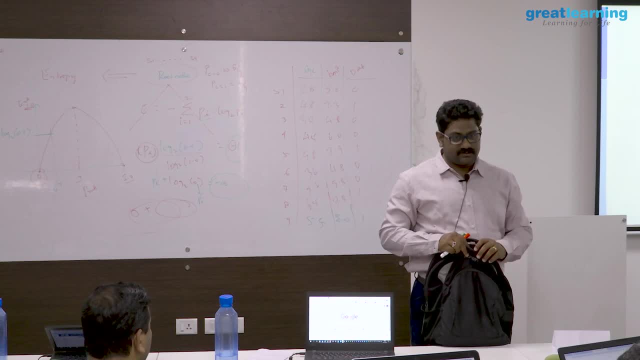 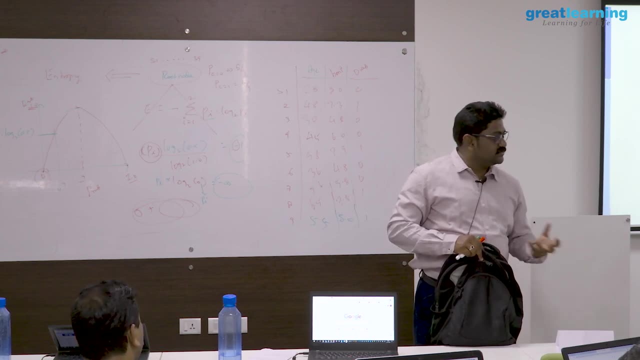 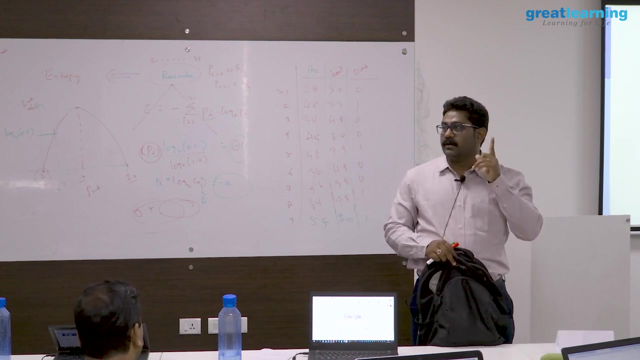 initially. now I keep eight red balls, two black balls. I'm asking you to pick the red ball. the probability of getting the red ball is high right and certainly level decreases if I keep all our red balls. what is the probability of getting red ball? hundred percentage one. what is log base 2: 1. log 1: 0. entropy 0: there's no. 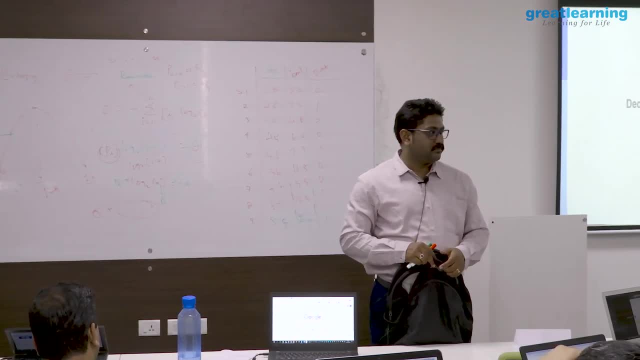 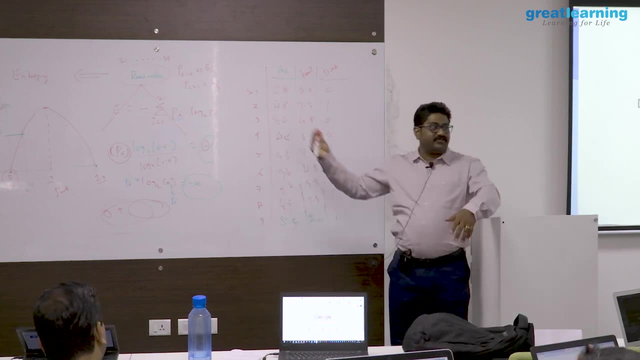 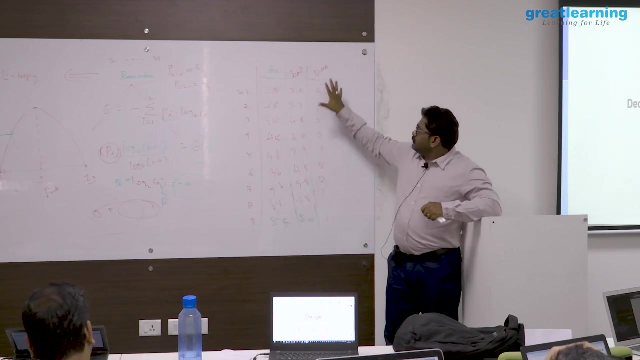 uncertainty. there is no confusion in selecting a red ball because all are red. similarly, if my record all are belongs to one class. why we need a classifier at all. we don't need a classifier at all. even I forget about classifier, even without classifier with this records, if at all, if I want to classify all my 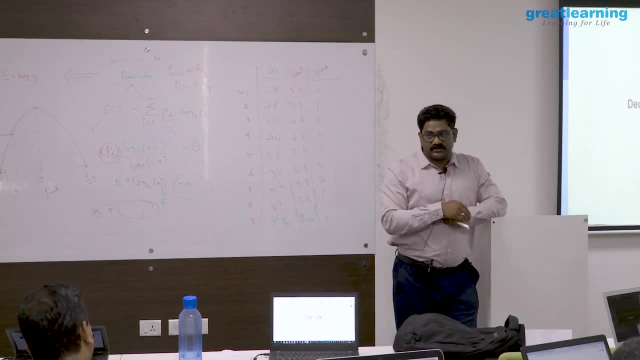 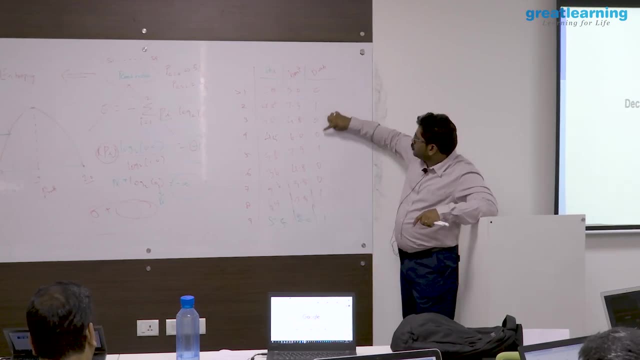 records either 0 or 1. which one do you prefer, 0 or 1? I check, I just check how many which is dominating? 1, 2, 3, 4, 5, 5 zeros against 1, 2, 3, 4 ones. simply, I say all are 0, 0, 0, 0 my. 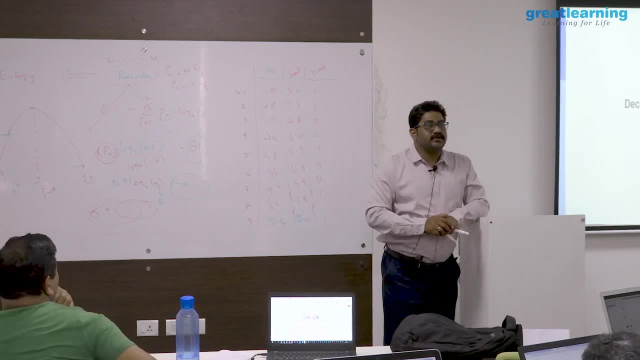 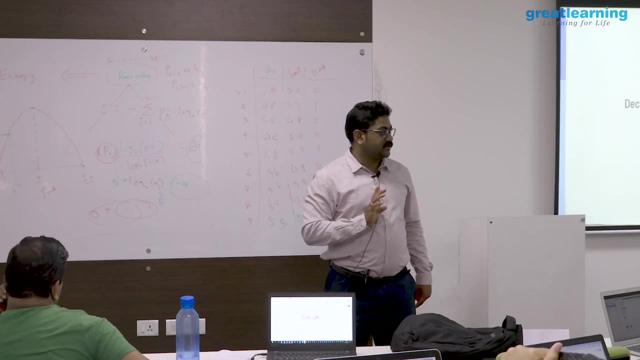 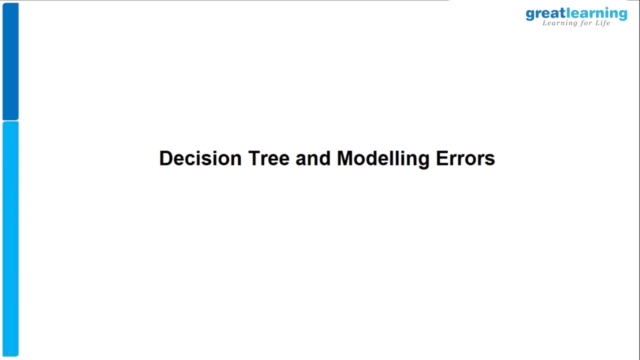 model. I'll predict all 0, 0, 0. I'll calculate model accuracy. what will be my accuracy? 5 records out of 9 records are correct. 5 records out of 9 records are correct. that is my overall accuracy, even without any classifier. that is called baseline model. even without building any model depend upon. 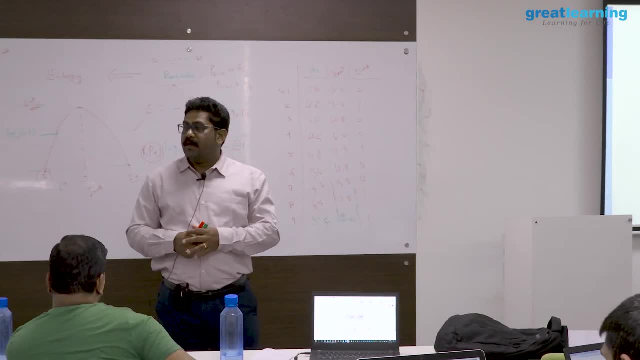 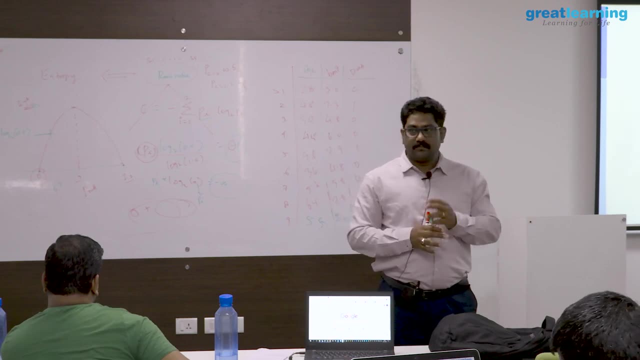 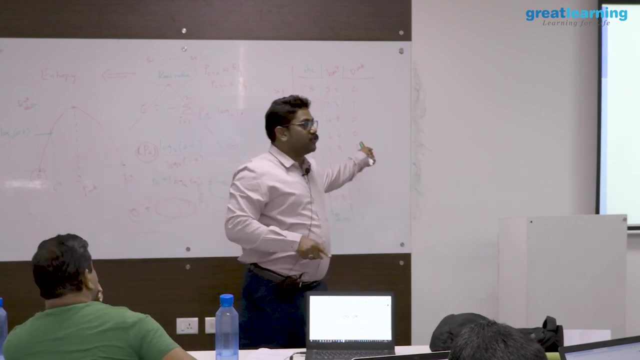 the nature of your classes: number of zeros and one based on the class probability. if I decide, all my records belongs to this class. of this class, you will get a fundamental score, right, basic level score you are. on top of that, you are going to build some ML model. your ML model should outperform the score. it. 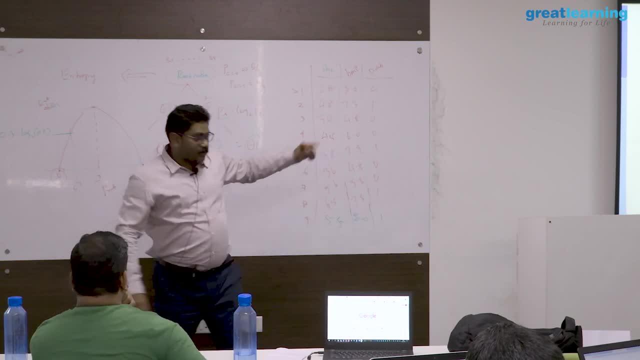 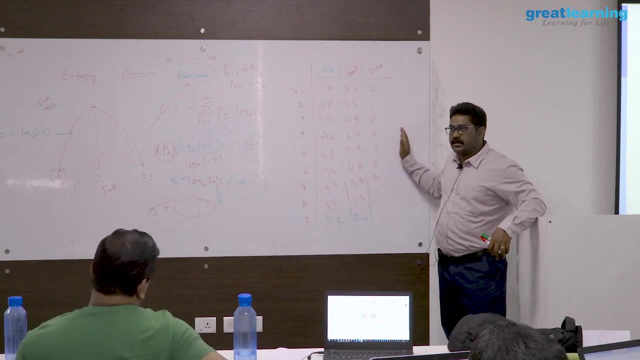 should beat the score with probability itself. I can say 0, 0 is all records and you are getting 60. let us say it's giving 60, 55 percentage. my base level score is 55 percentage. on top of that, you are building some model and your model. 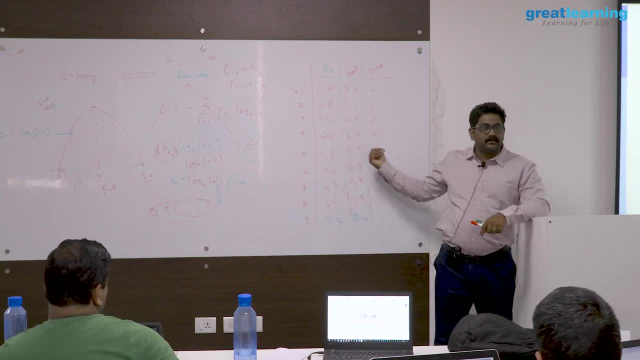 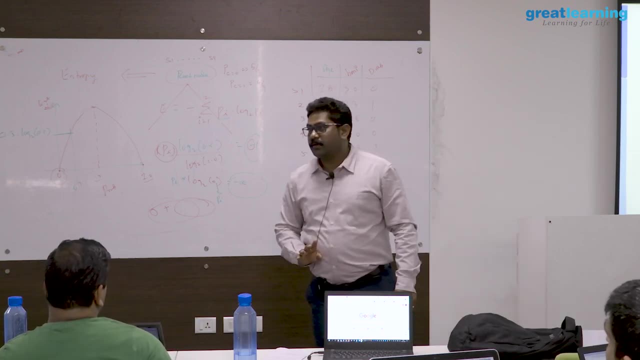 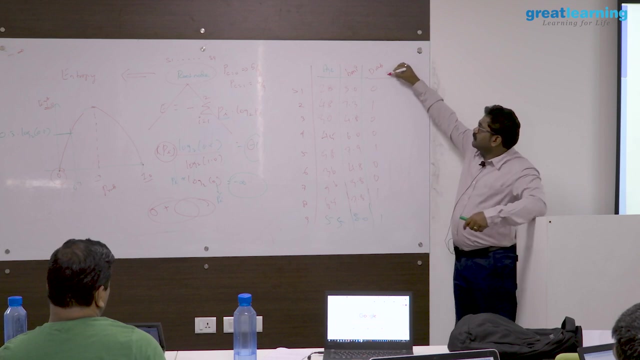 should not say 50 percentage. your model is worse than was then probably score itself. so always keep this as a benchmark. if it is a regression problem, what is your base level score if it is a regression problem, instead of diabetes, if I suppose if you have a glucose level, glucose level, let us say 250. 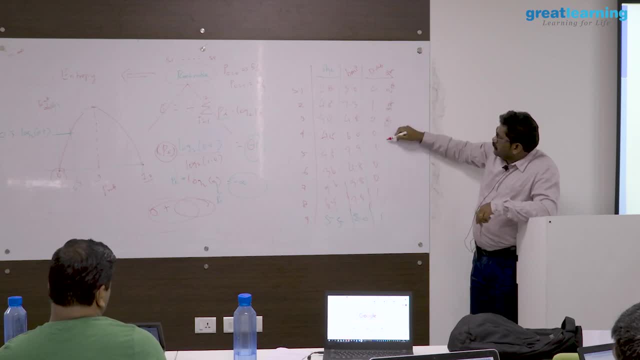 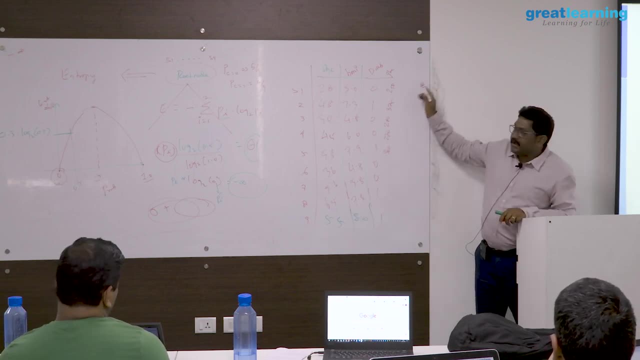 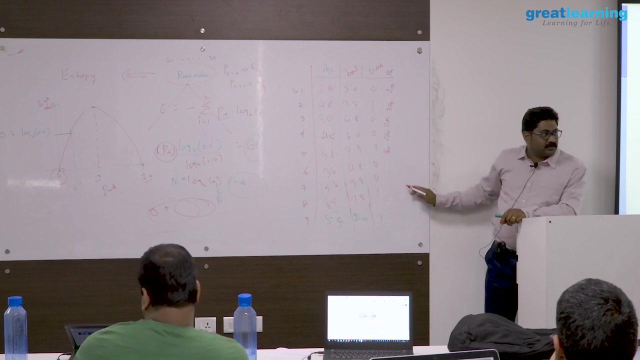 for him this is 375, is a score: 280, 270, 360 and so on. I just simply calculate the average for all the records. I will be predicting average average, average average. all the records will be predicting as average score. you have the actual and predicted as average. actual is Y and Y average, Y minus Y, bar you. 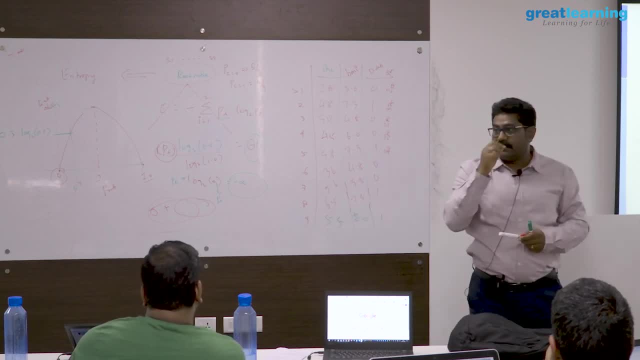 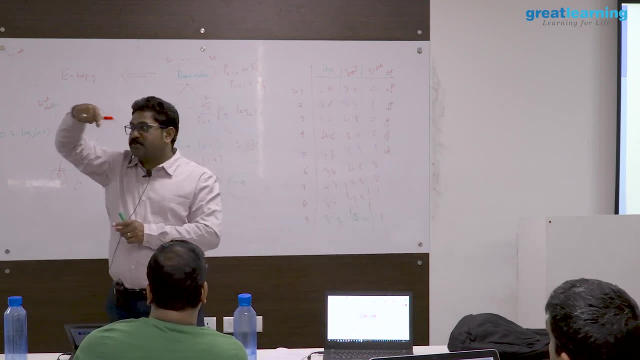 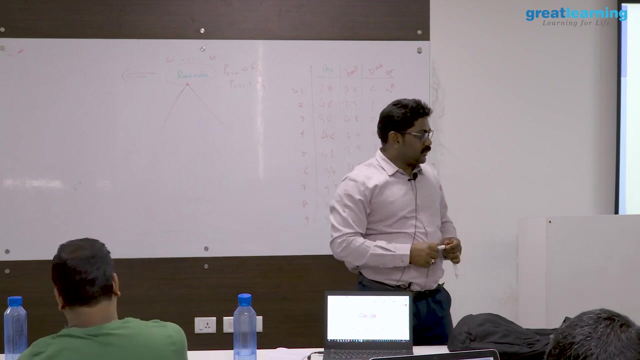 calculate the differences that you will get a RMSC score right. that RMSC is a base level score. on top of that you are going to build some regression model. your- your regression model score should be less than that baseline score. hold the methodology in many business problems: decision tree. 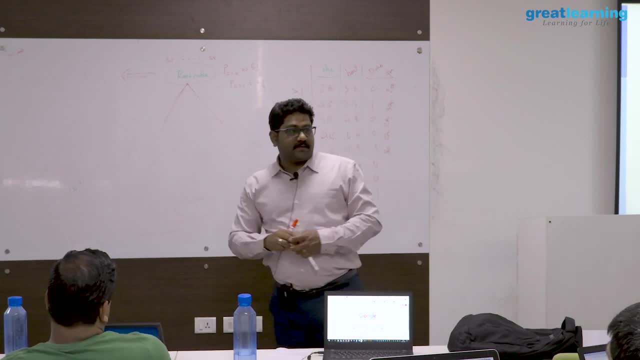 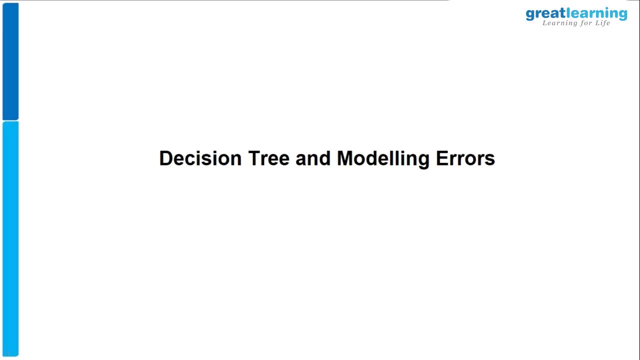 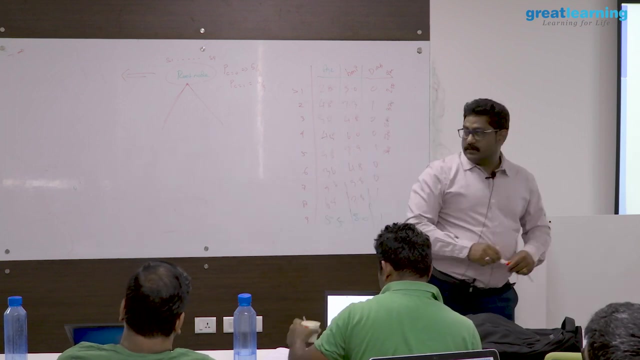 based or business management technique. we have used this decision right. so what we ask at the root node? you are using some parameter and you check the RMSC how you really can build some model. so your thing, you will be thinking before any discussion right now, you need to build some model, so you need to check your model. what the the 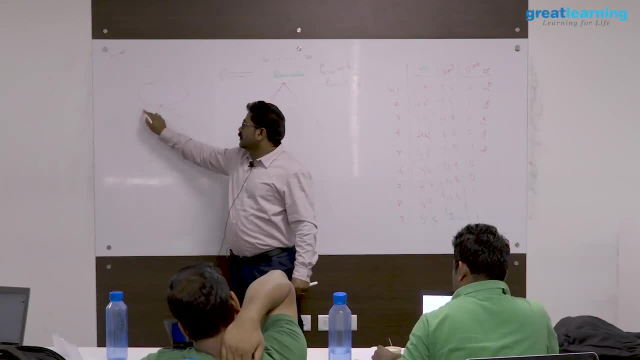 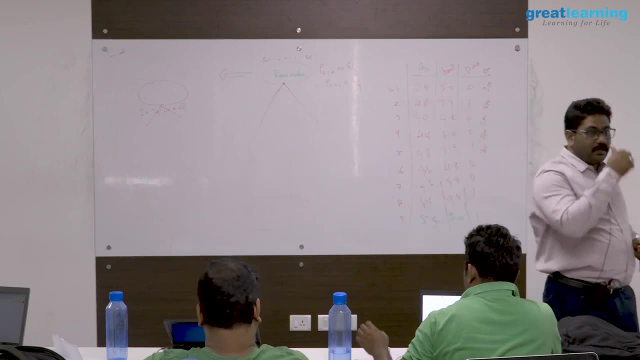 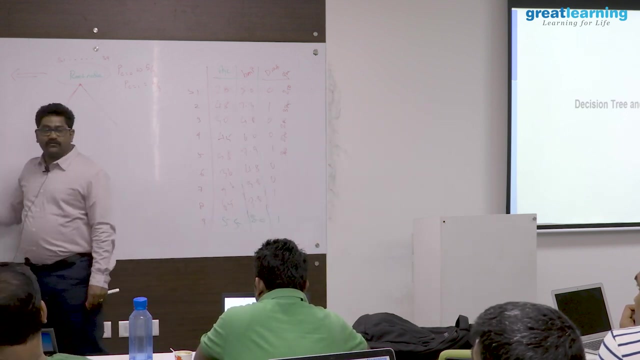 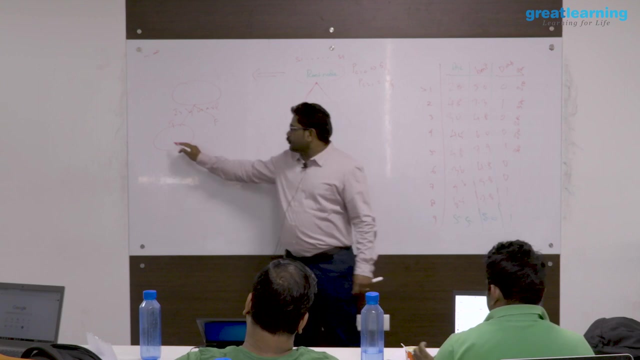 end product be this model-like modelサンダ Film, even our initial 30 minutes of discussion. suppose you want to build some model. you have true or true or false, like a flowchart. if Y is available, what do you do? decision you take. it's a supervised model. supervised false means it is. 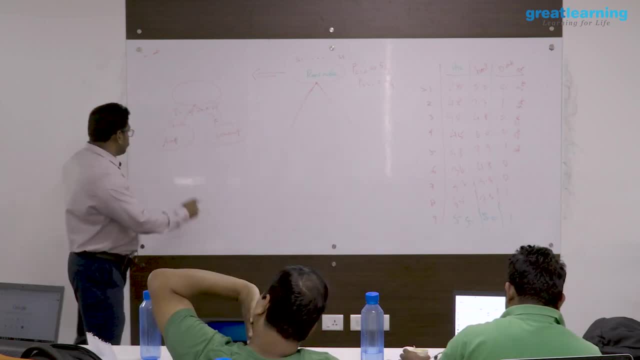 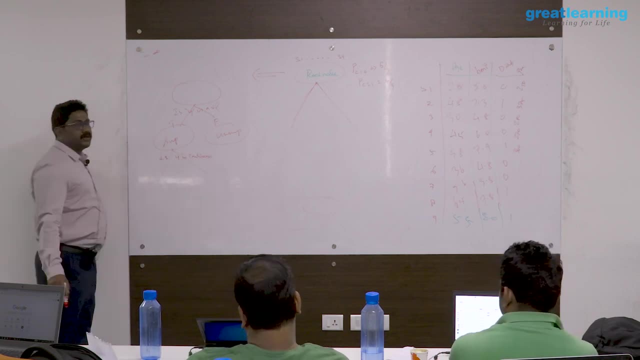 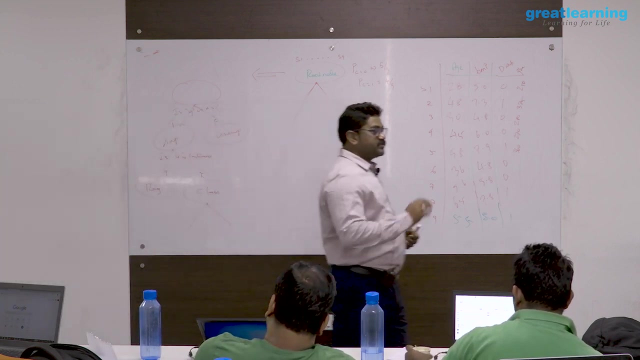 unsupervised model. and again, here we're going to ask another condition. condition is: Y is continuous, continuous numeric? again, you have true, false branch. if it is a continuous is true, you're going to build a regression model, false classification model. again, you can ask the classification model, you can subclass, categorize it for. 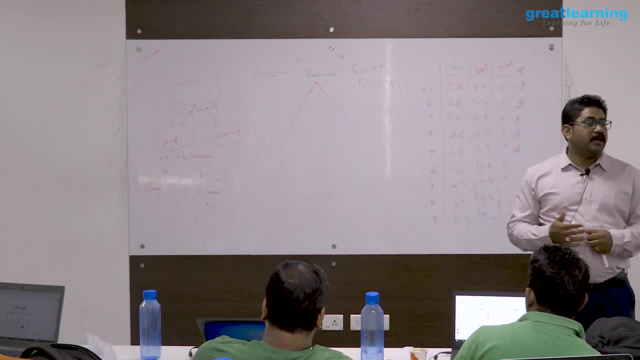 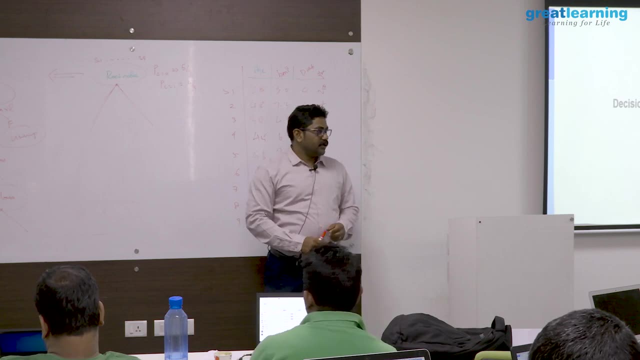 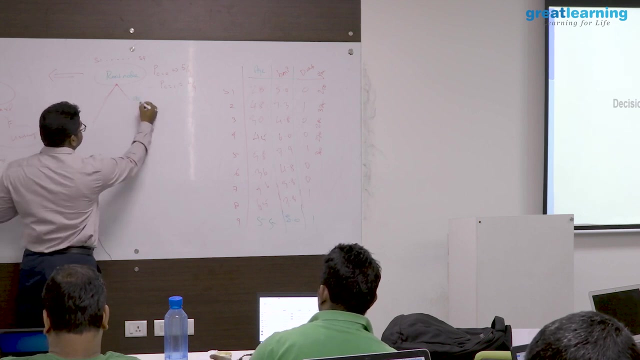 simple decision-making itself, your decision trees, whatever the day-to-day life decision-making. we are using this kind of for branching out: yes, no conditions, true, false conditions. the same logic we are going to apply here. here, let us say, if I'm going to start with each, each parameter, why age? why not BMI? 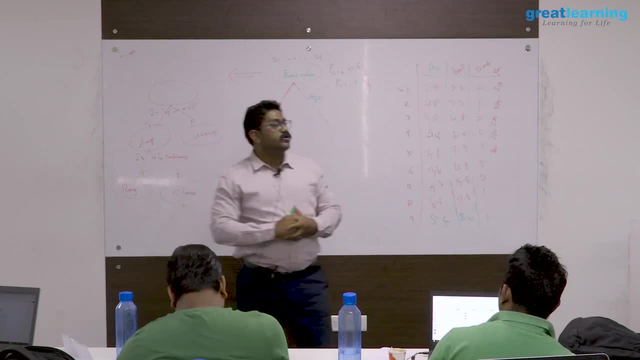 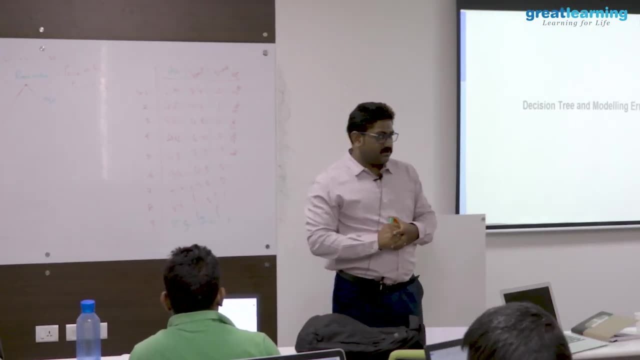 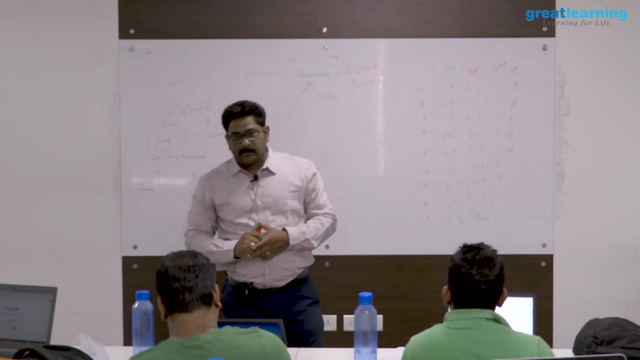 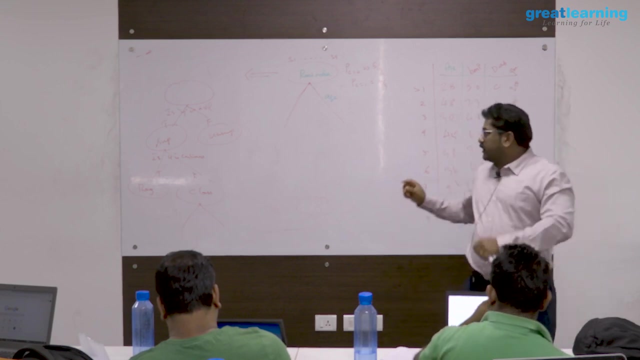 your model will decide. we don't have any control over it. decision tree classifier is also called as the greedy classifier or greedy algorithm. why it is called as a greedy algorithm? let us say your data set has three classifiers. let us say your data set has ten attributes out of the ten attributes. first it will check, if at all. 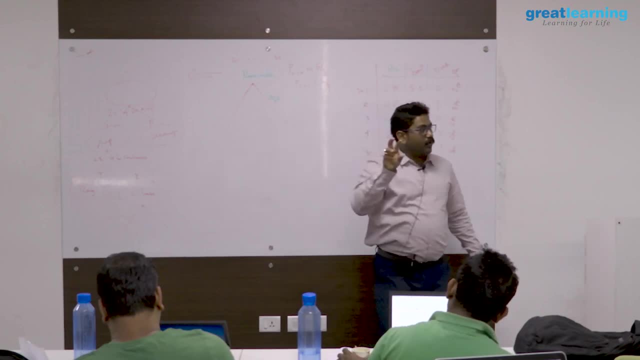 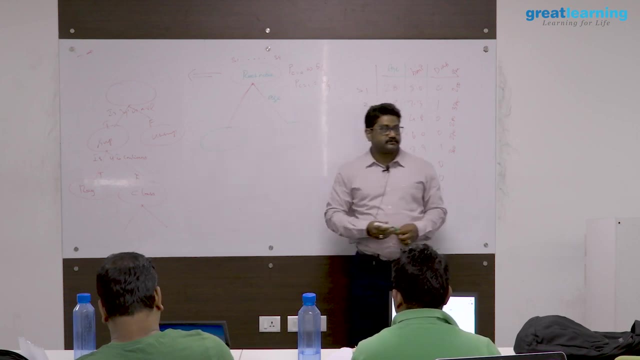 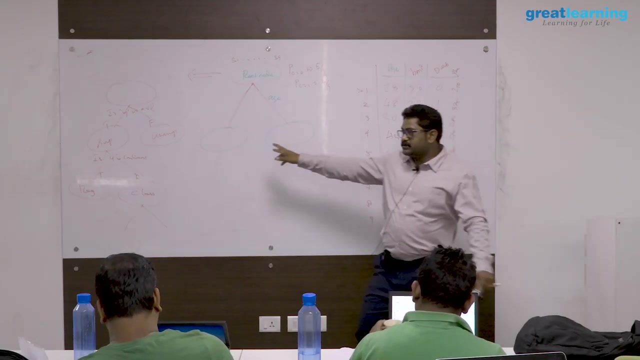 if I want to branch my initial branch out with attribute number one, okay, definitely. certain records are going to be collected here. certain records are going to be collected here, if at all. if I want to use a different attribute- the number of records collected in this branch- it will be different, definitely. 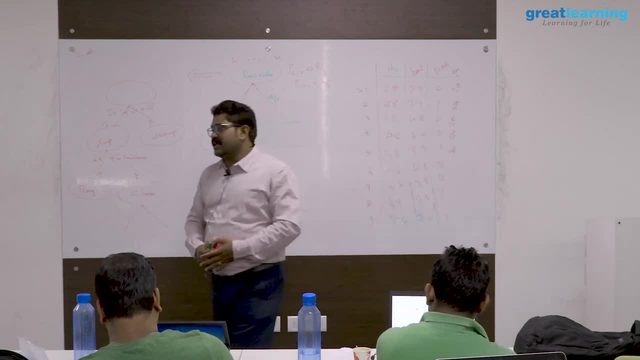 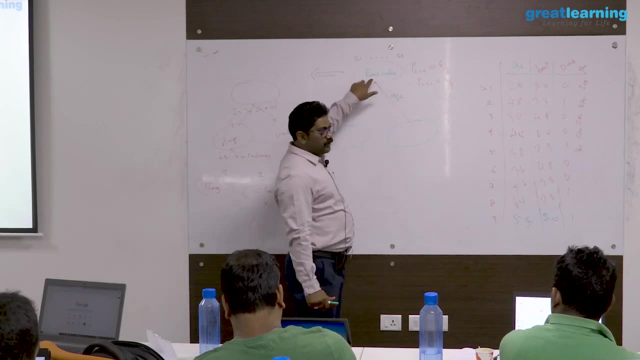 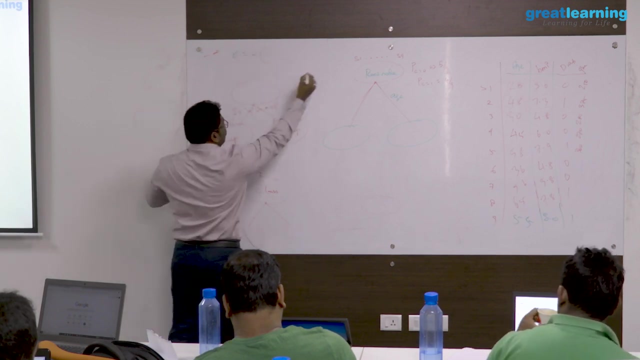 right. so how do you validate the split, the effectiveness of the split? how do you check the effectiveness of the split at the root level load we calculate? we are going to calculate entropy. can you please help me in this calculation. how do we think? let us calculate the entropy equal on to. i take minus sign outside. 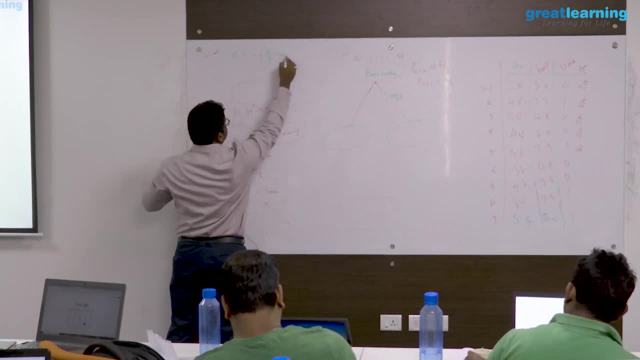 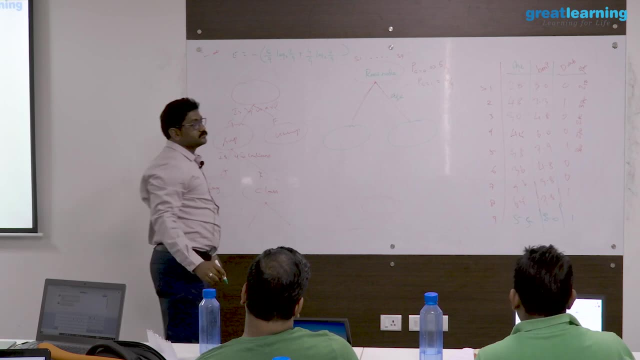 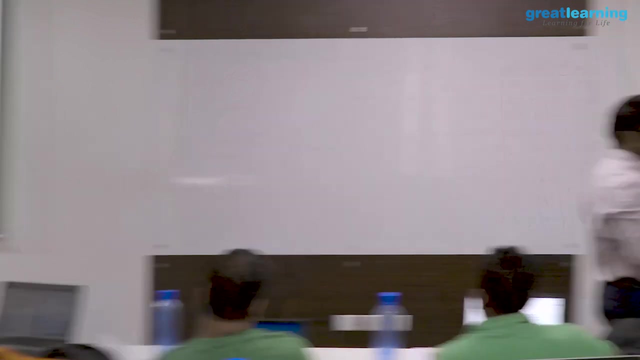 please calculate and tell me: five by nine, log base to five by nine, plus four by nine, log base two, four by nine, you will get something close to point between. you get something close to point between 0.85 to 0.9, something you will get that is the entropy level at the root node, the minus. 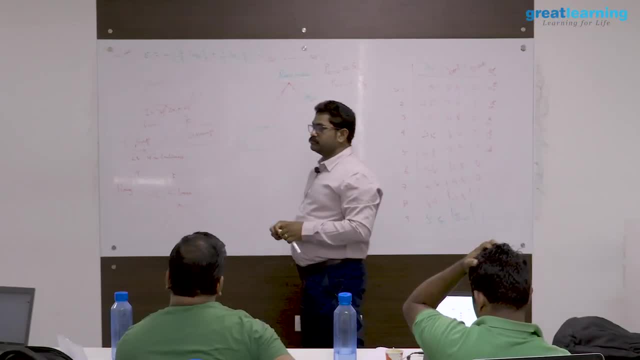 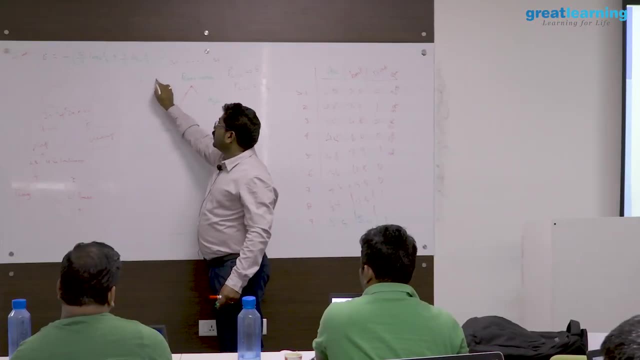 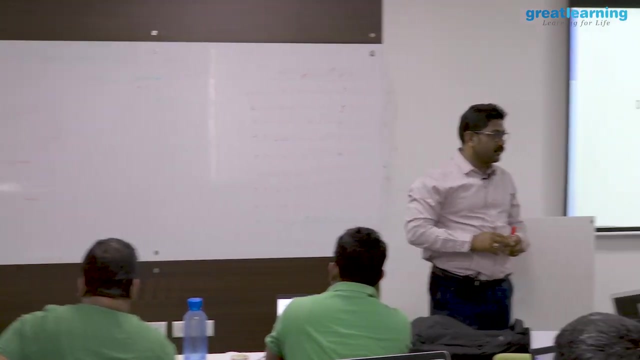 sign will cancel it out. I think this sum, you will get minus sign and this minus and minus will cancel it, you will get the positive entropy score. okay, 0.98. that means almost close to 1, right? when do we get exact one? 50-50 percentage, 50 percentage, 50 percentage. 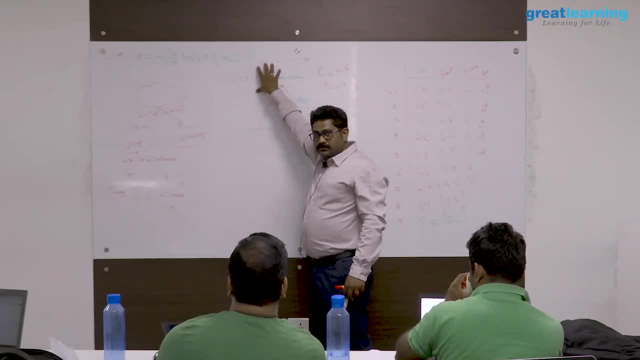 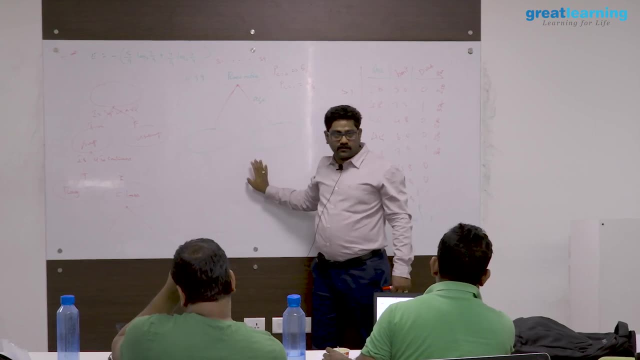 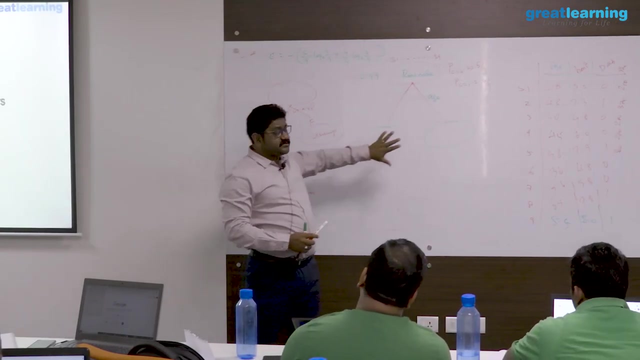 so 0.98. my entropy level is high, so that means there is a good reason to split. we have very good reason to split. because it is a highly ambiguous, I want to split my records. After splitting the records, on what basis I can test whether the effectiveness of the 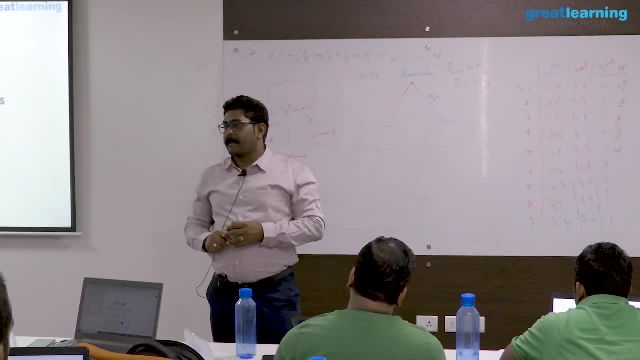 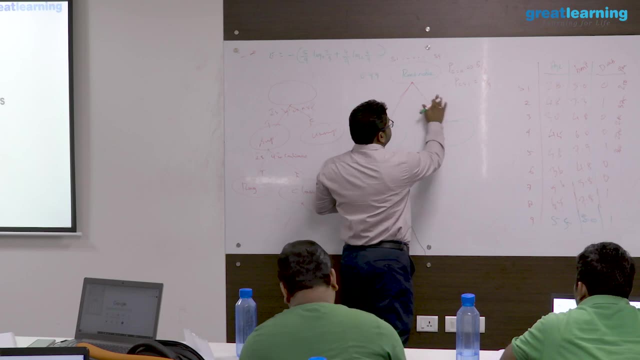 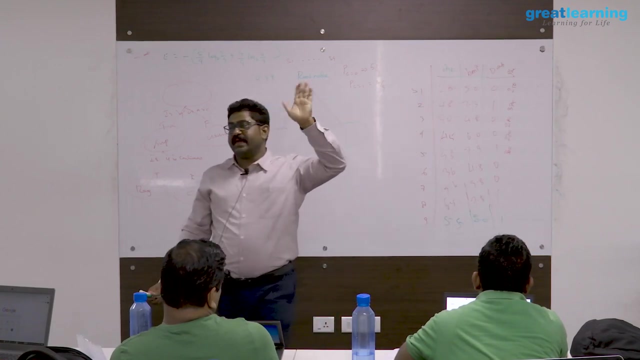 split, how we can cross check the effectiveness of the split. okay, let us apply some split based on the age as a criteria. So let us fix some threshold value for the age you can. can you tell me by, just by visual observation, you just tell me: let us say, above this age, we will say diabetic below this age. 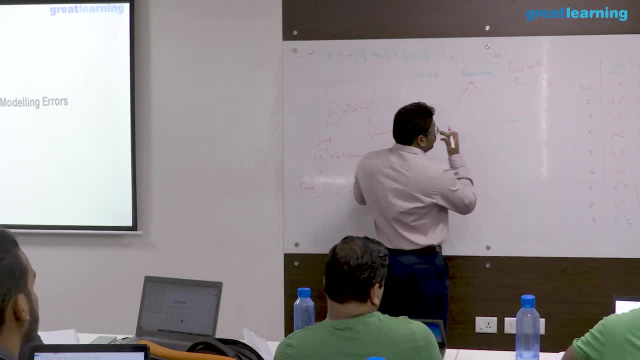 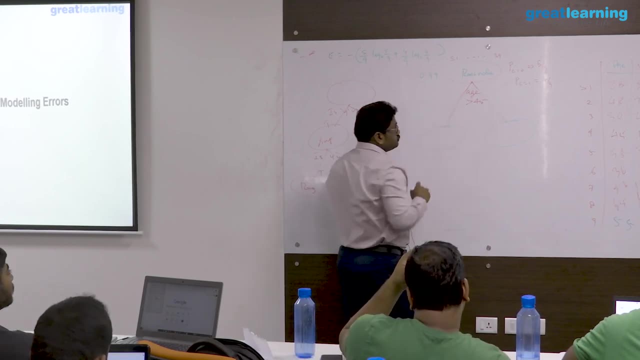 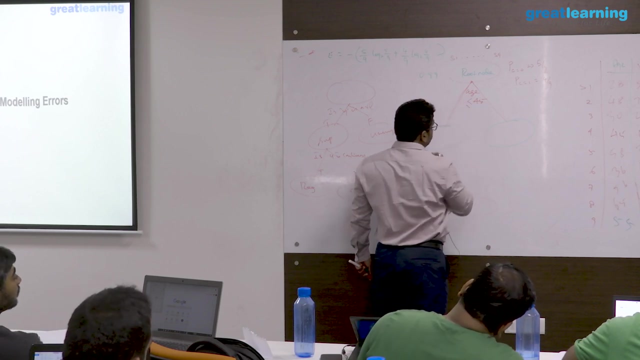 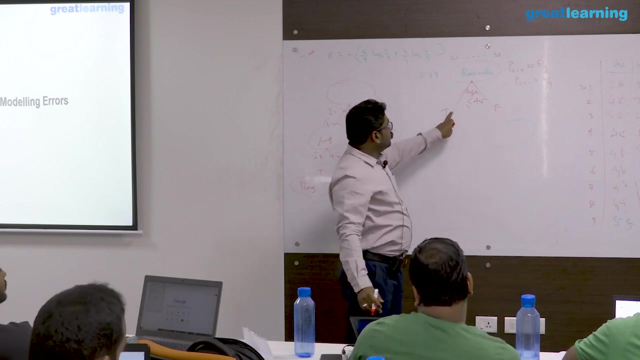 no diabetic, okay. So I am going to make a condition: age greater than 45- okay, age greater than 45 is diabetic, okay. otherwise, less than or equivalent to. If this is true, healthy- Okay. This is a true side. this is false side. true, it is not a healthy diabetic. I am not coming. 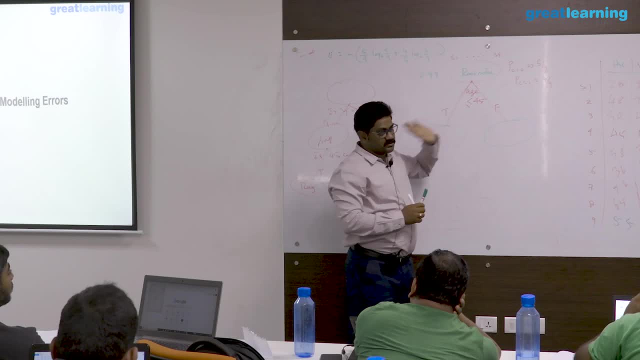 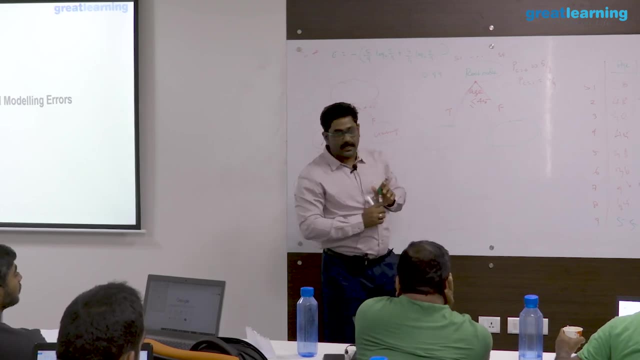 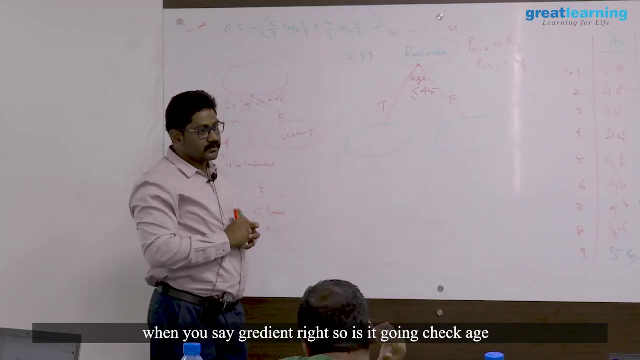 to that point only I need to check true or false. I have not come to the conclusion. if all my records here are healthy or diabetic, that conclusion you have not arrived so far. So, based on this condition, When you say greedy right, so is it is going to check age, BMI, diabetes? sorry, not diabetes. 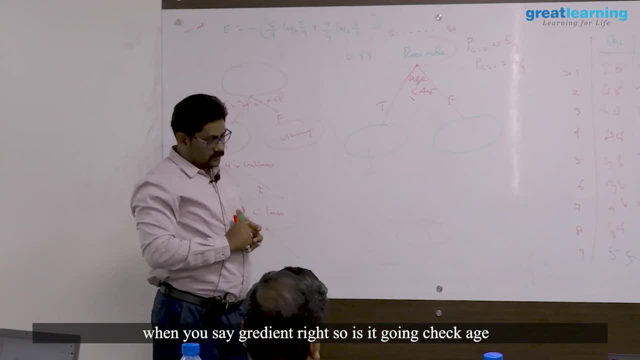 age, BMI, diabetes. Okay, Okay. So this is the age and BMI go Go which are having the more entropy. that one you will see like That is what I am coming back to, that point. I will justify that point after splitting this. I have a question. 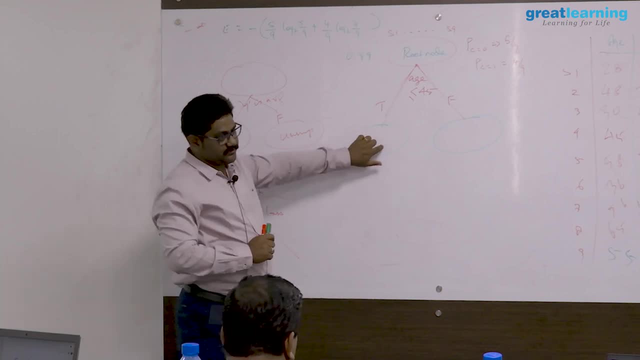 Yeah, please, We are. we are splitting it because it is greater than 0.5.. Which one The at the No, no, no, no, not greater than 0.5. some value, Okay, Some higher level of entropy, right Closer to 1.. 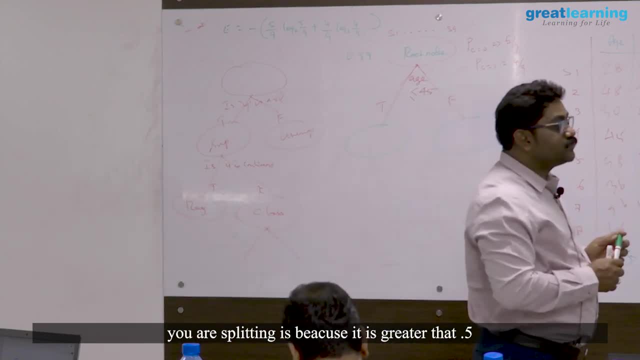 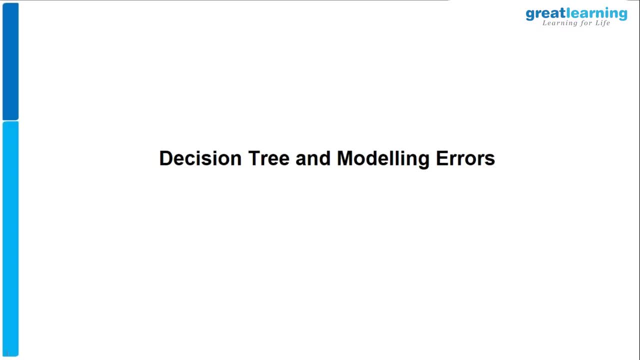 So it is greater than 0.5.. So it is greater than 0.5.. Some value Some higher level of entropy, right Closer to 1.. If the entropy level is very less, let us say 0.1 means all are belongs to one class more. 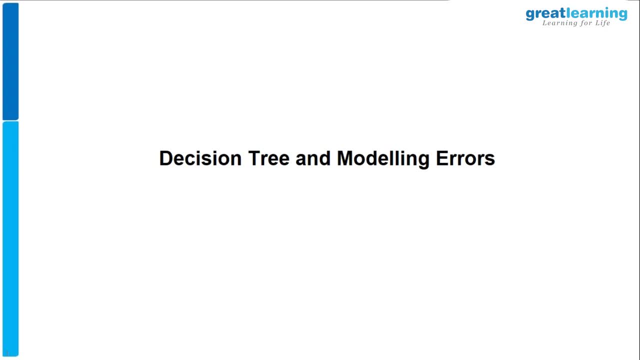 or less all your records belongs to one class. there is no need to split it. When you get that pure class, only at the leaf node, you start to the root node and finally you branch down. finally you go to the leaf node- because it is a pure leaf, all the records. 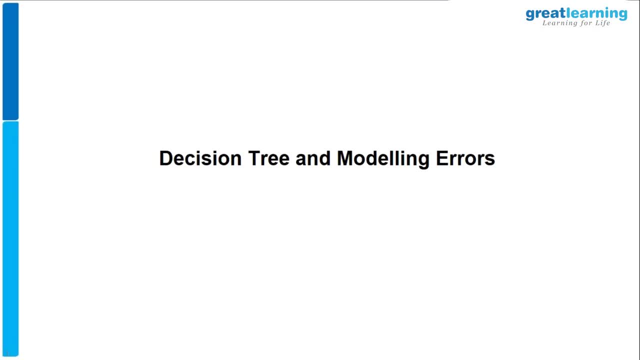 to only one category, that is, a pure leaf. what is the nature of pure leaf? all are zero. what is entropy? entropy zero because all are zero means probability of picking zeros. hundred percent, age: one log base to one zero. entropy zero: once the entropy zero you start splitting. 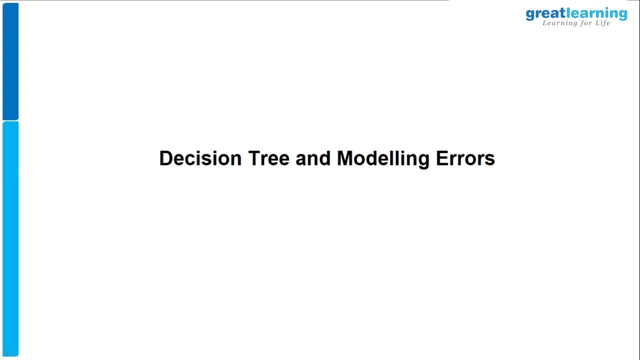 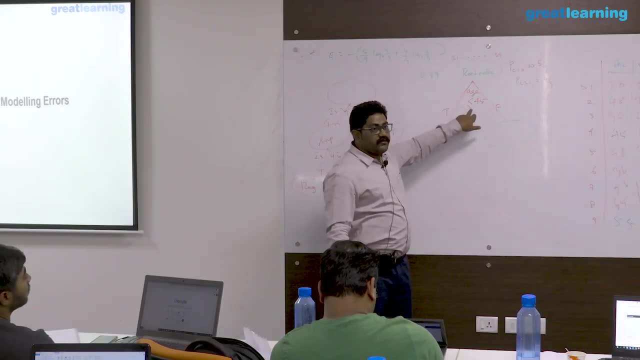 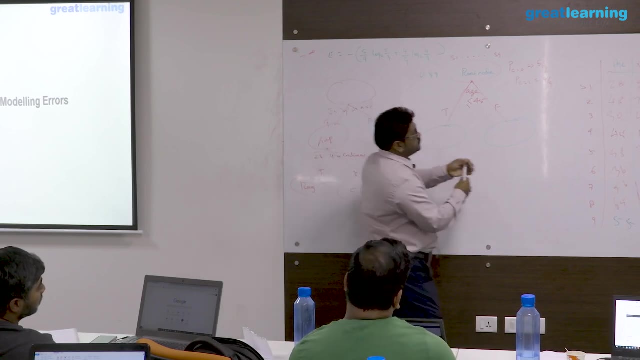 you stop your splitting, your tree will stop growing further. that is a stopping criteria. ok, we will come to that. so, if at all, if it chooses this as a threshold and tell me which of the records will come this side, what is the record now? first, you will look at only 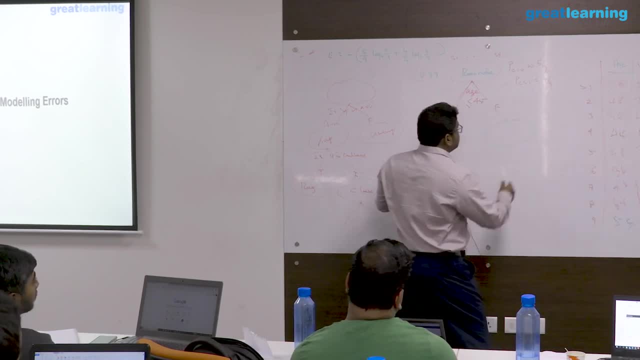 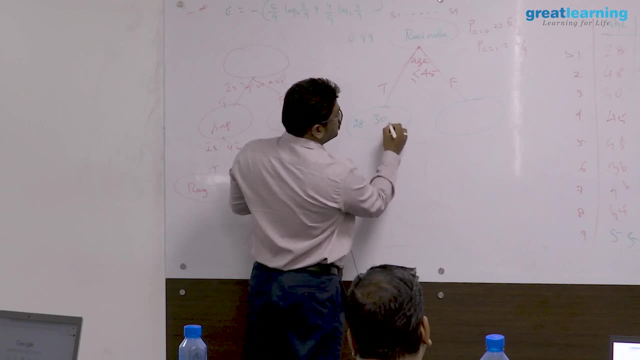 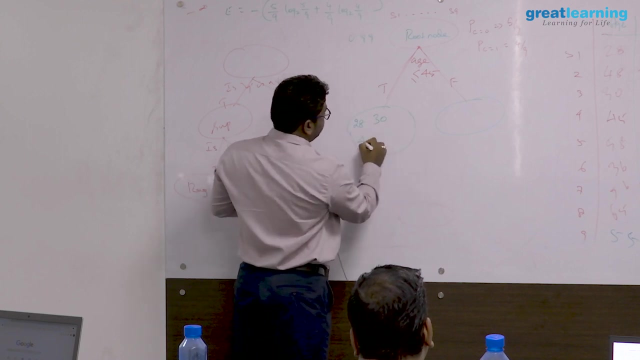 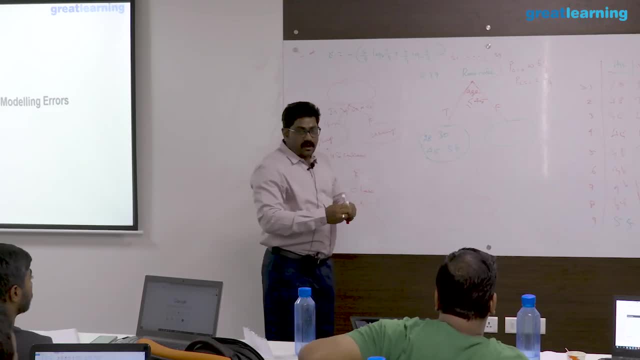 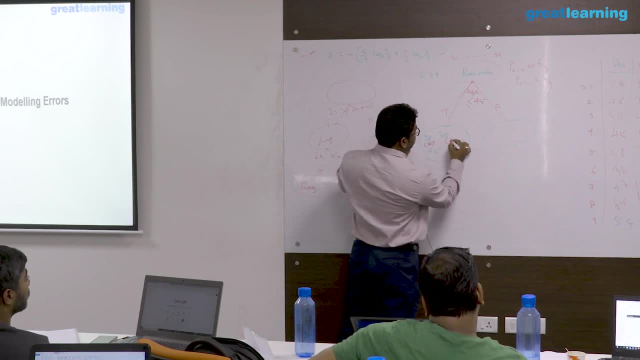 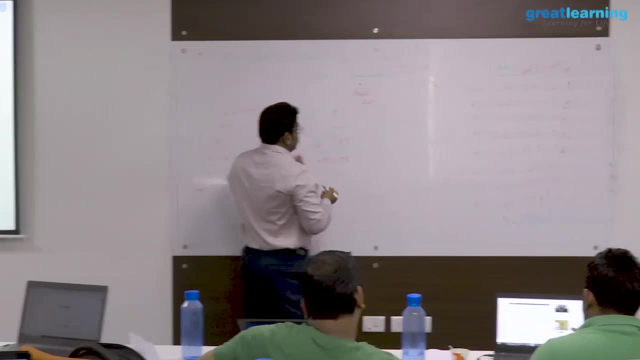 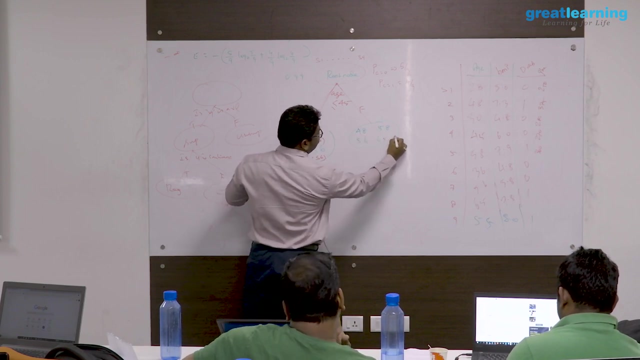 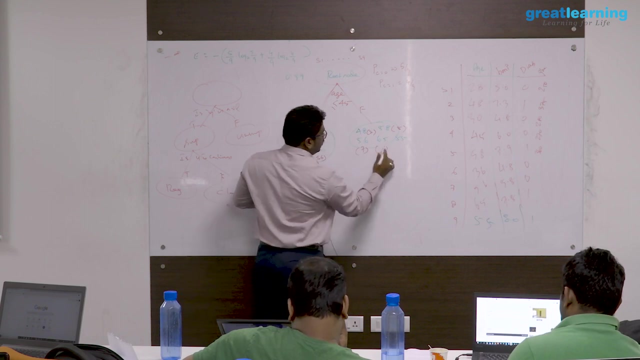 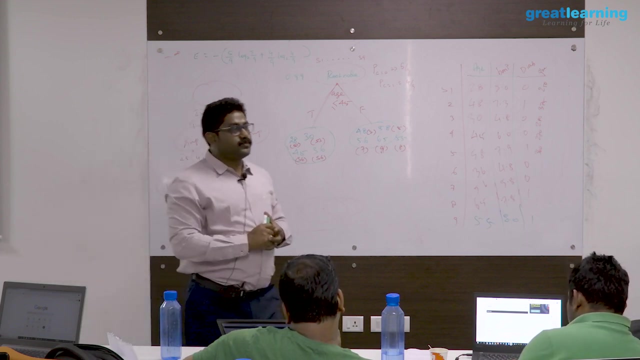 twenty eight. record number s one. ok, this is s three s four, this is s six, forty eight, fifty eight, fifty six, sixty five, fifty five. 2, 5, so this is 9,, this is 8.. Decision tree is a supervised or unsupervised? 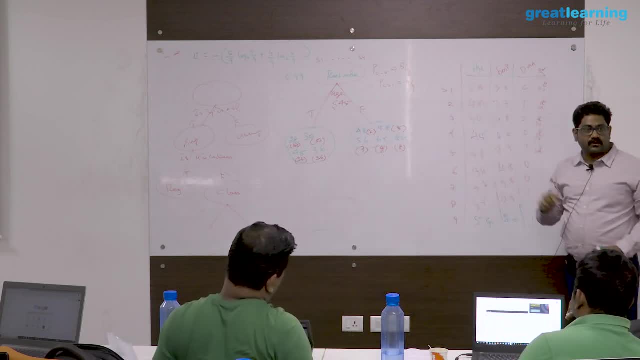 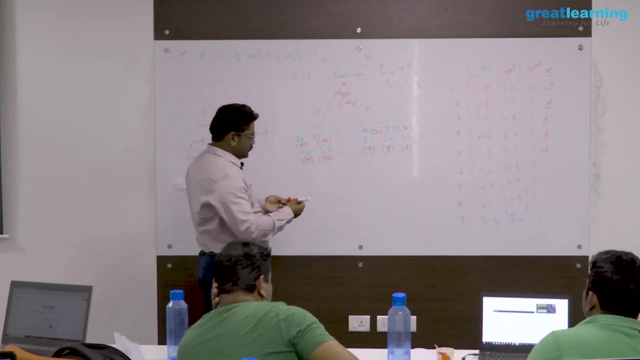 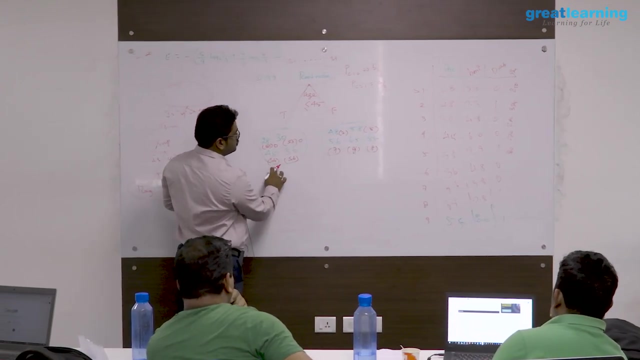 It is a supervised learning. that means we have the known labels for each record. Now you attach the labels. what are the labels for S1?? S1 is 0, S3 label 0, S4: 0, S6. At. 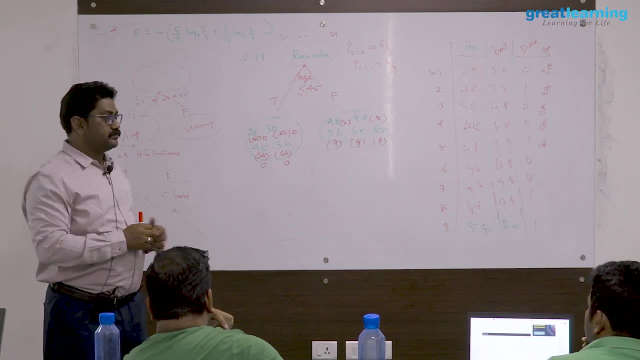 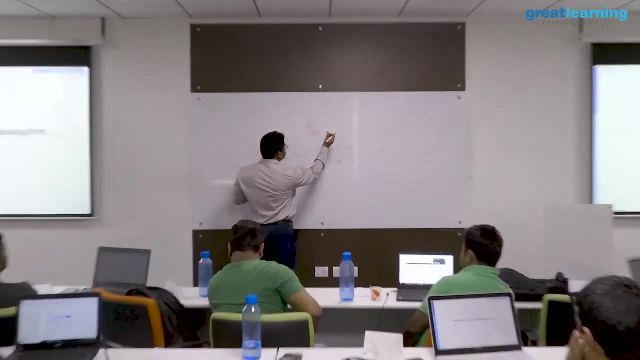 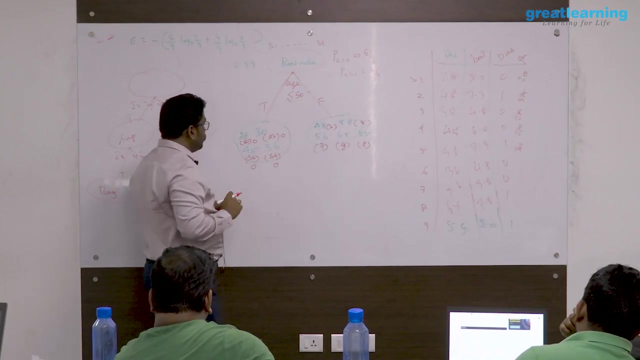 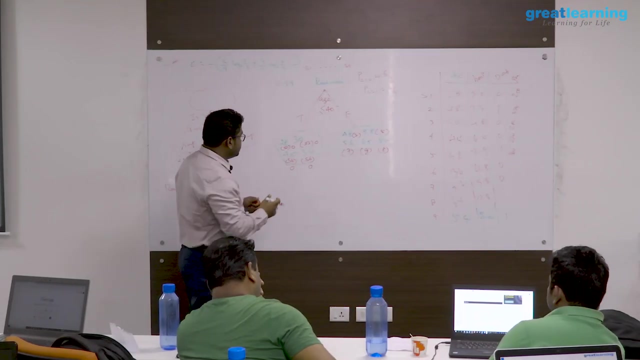 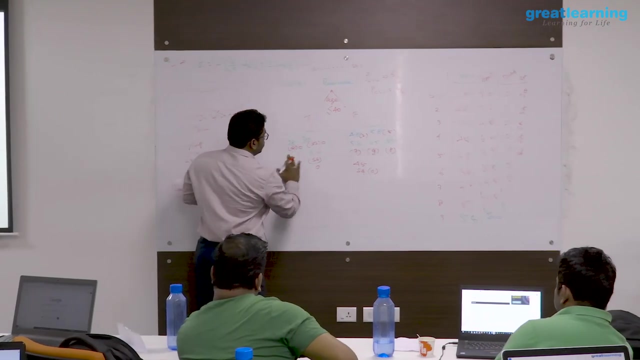 the first level itself. you achieved pure purity at first level itself. Sometimes, sometimes, let me change my threshold value. sorry, less than 40. I will keep less than 40.. In that scenario, 45 will go here, am I right? 45 will go here. this is S4, the label is 0. Because 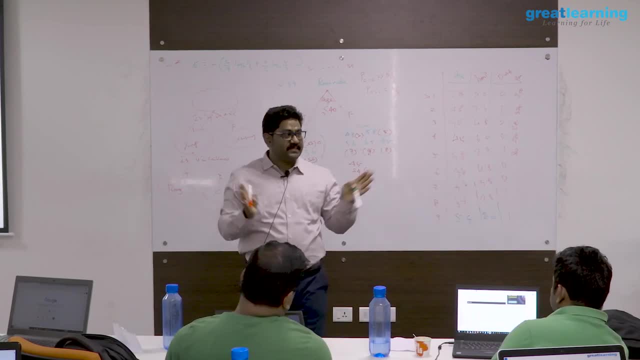 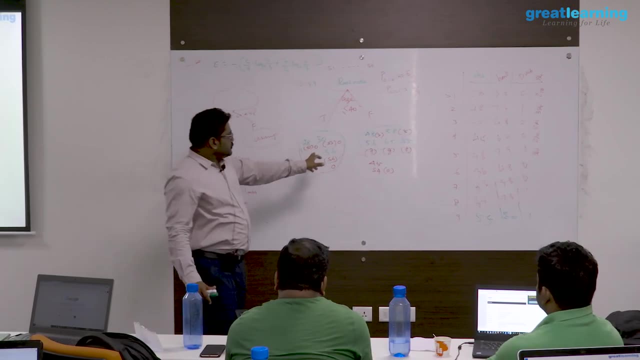 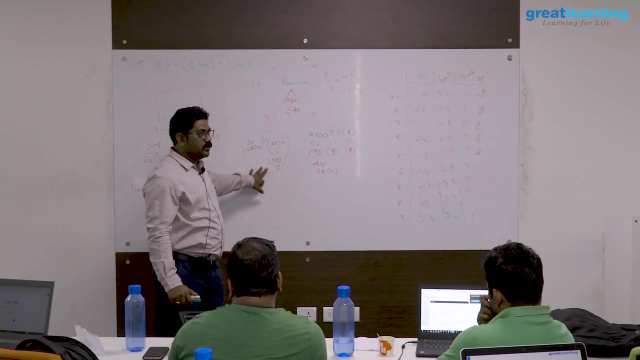 I have given so simple values so that it is a linearly separable. but in your reality your data won't be looking like so linear, simply linearly separable. Definitely there will be a mix. So here you have again. you have all belongs to 0, this is a pure leaf. 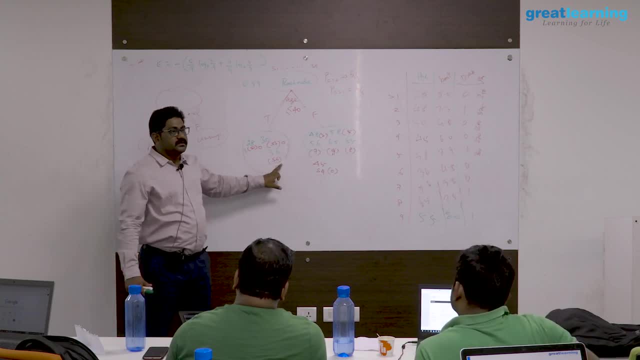 right, this is a pure leaf. all belongs to. you can declare: S1, record 0, S3, record 0, S6, record 0,, 100 percent. What is the class belongs to all these records? you can say it belongs to class 0, because which probability is high? 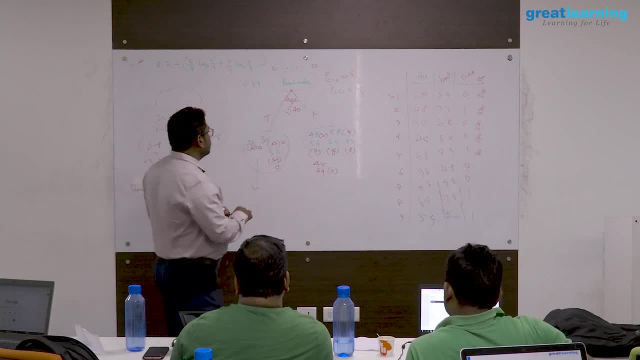 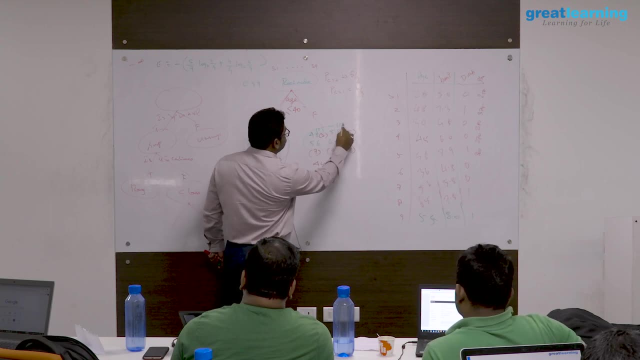 Class 0 probability is high, am I right? Class 0 probability is high. Same way, how many 0s and how many 1s here we have? Ok, this is 1,. this also 1, this is 1, 1, 1.. Ok, 56. 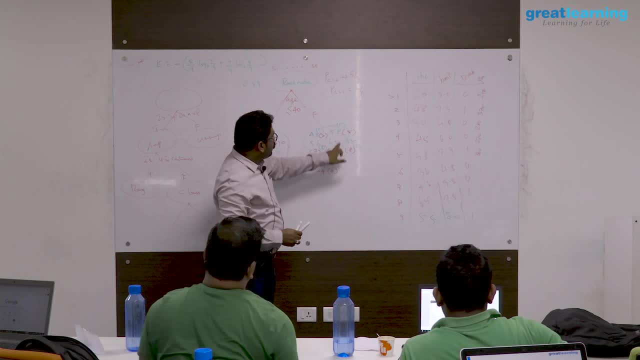 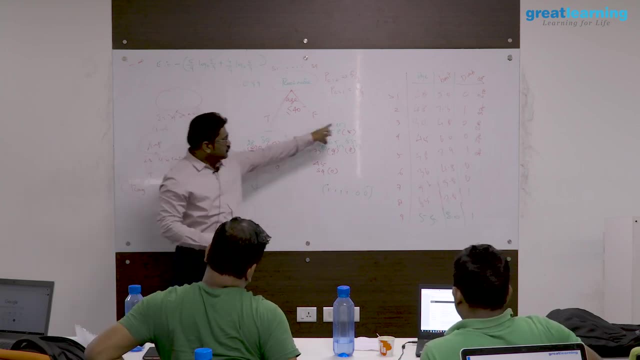 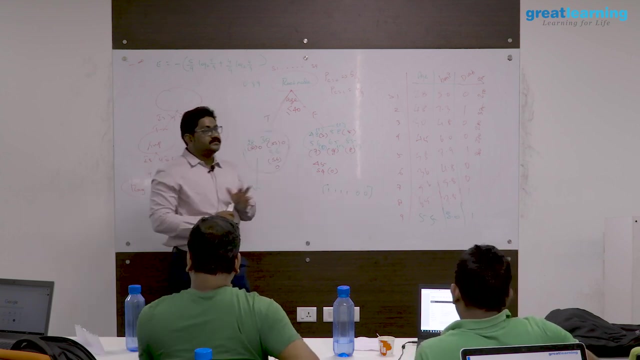 is 0. There are 2 0s. I have 4 1s and 2 0s. At this, at this node, I have 4 1s and 2 0s. What is the probability? which probability is higher here? Class 1 probability is higher. 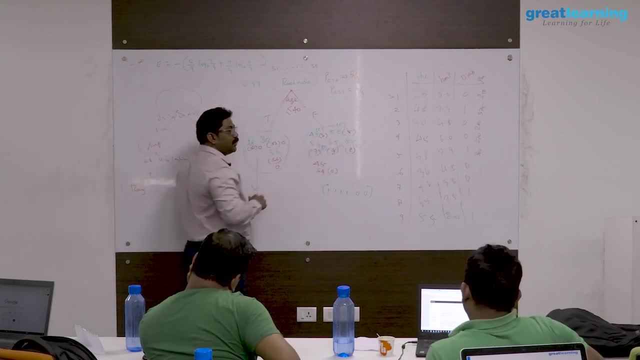 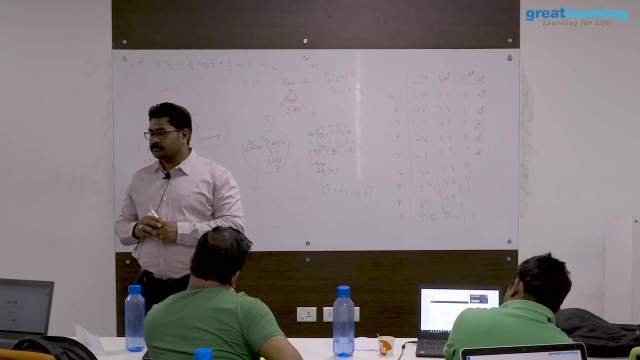 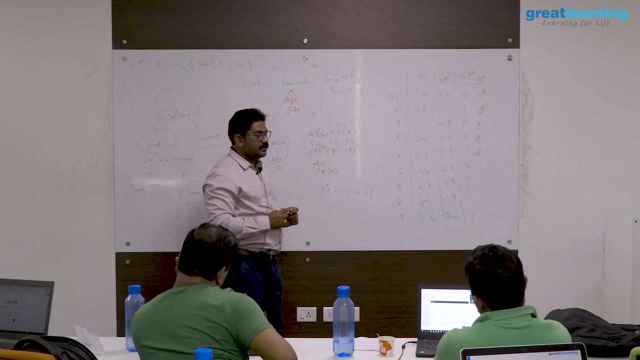 that means all my records, all my records. I will attach label 1.. Whichever probability is high, I will be attaching that as a label to all my records. If I attach all these records 1, how many are correct classifications? how many are misclassified? These 2 are misclassified. 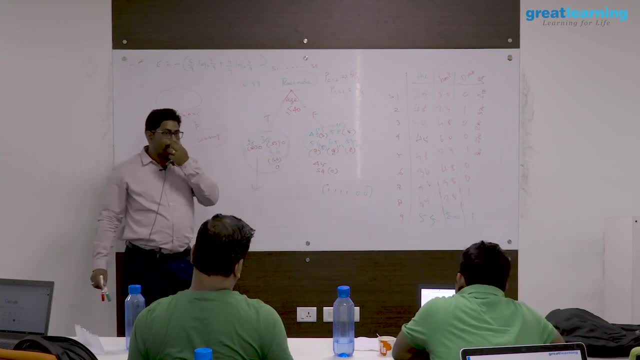 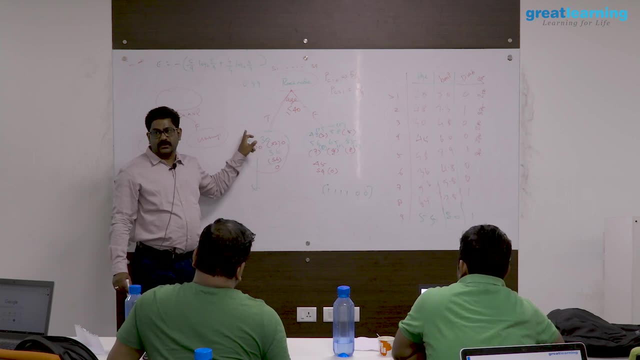 these 2 are misclassified. these 4 are correctly classified Here. all 3 records I am attaching, because the probability of 0 is 100 percentage, All my records I will be attaching 0. Though if I have 1, suppose I have a label 1, there. 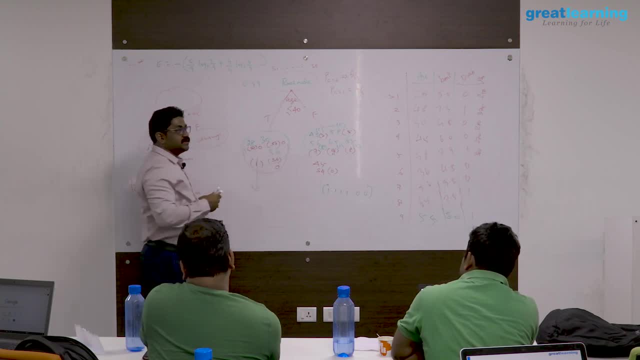 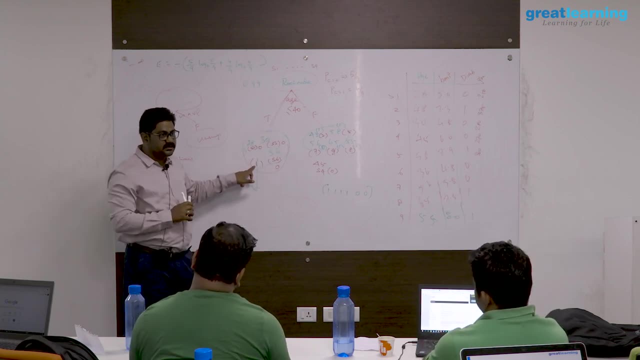 is 1 record 1 is mixed up here. still, my 0 probability is high, 3 out of 4, 75 percentage. The probability of class 0 is 75 percentage. probability of class 1 is only 25 percentage. 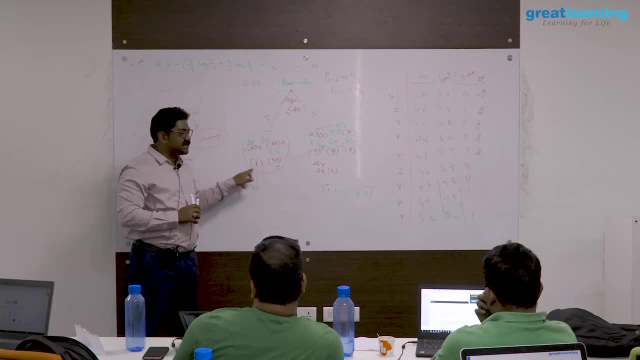 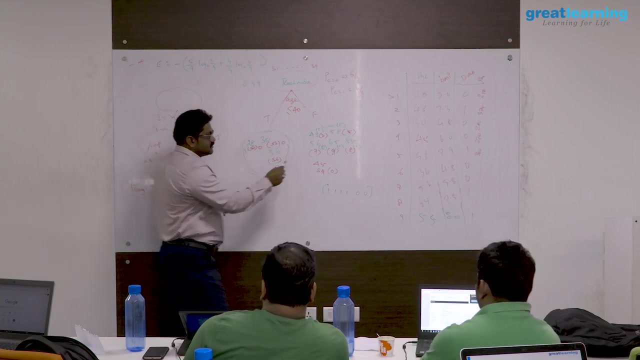 That means all these 4 records. I will attach 0.. This is misclassified, Though it is 1,. your decision tree will attach 0.. Ok, 0 for this record also. So So how do we justify this split? is good split or not? I need to calculate the entropy level. 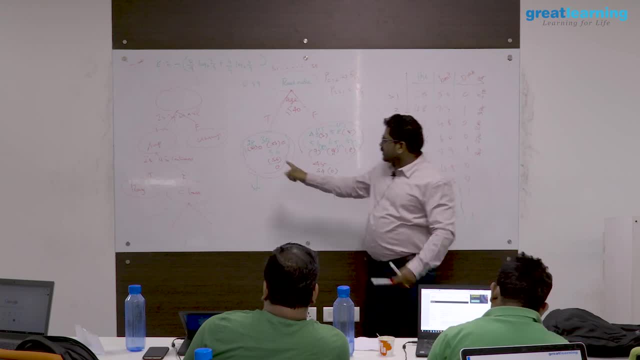 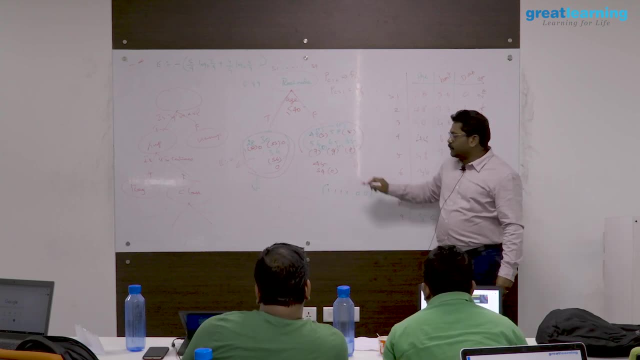 at this branch, at this node. Once again, I need to calculate the entropy level. What is the entropy level here? 0.. Entropy level is 0.. What is the entropy level here? 4 by 6, you should not use 9 here because it is branched out. 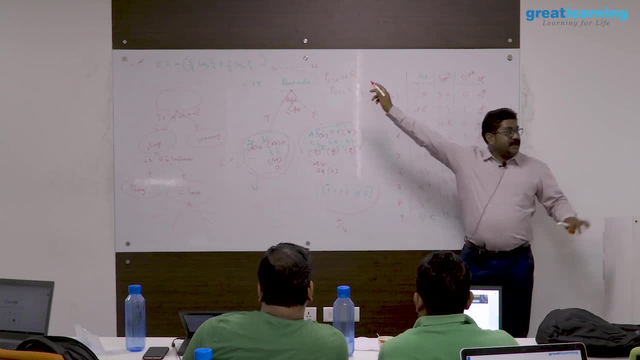 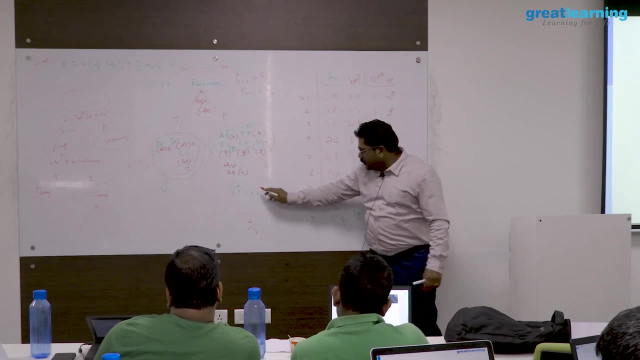 4 by 9.. 4 by 9.. 6 by 9.. 6 by 9.. because it is branched out from nine records. you have collected six records here. three records went there, so the probability of class one is four by six into log base two, four.